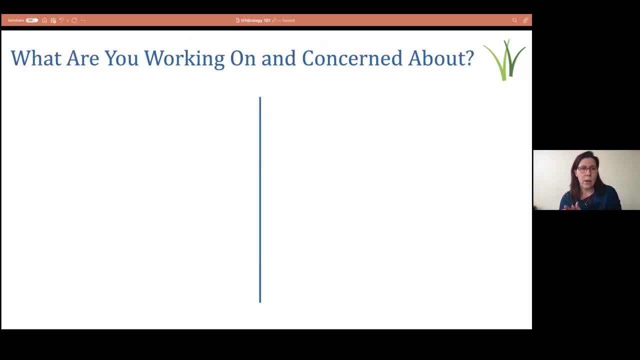 So I want to start with a little bit of engagement so I can get a feel for who's in the audience. It's like we have a great group here. We're going to run two quick polls back to back. The first one- I'll share what they are and then Chris can run them- is I'd like to know the top water management concern your county has prioritized in terms of. 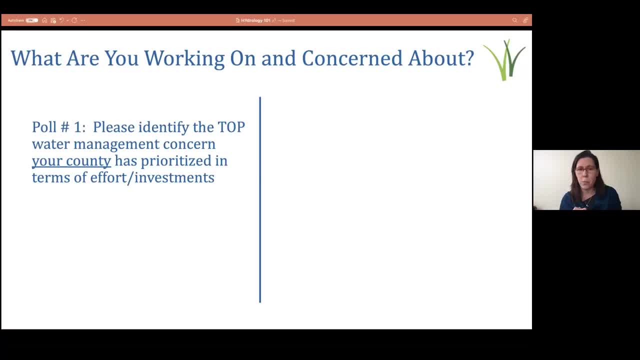 the efforts or investment you're making, and you'll see the choices when she runs the poll. And then the next question is: if you were making all the decisions and in charge of the money and the workload, what issue would you prioritize for new or increased investments or efforts? So, Chris, let's go ahead and run the first poll. 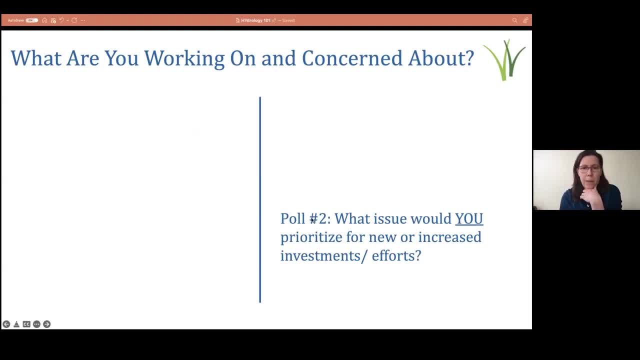 Here we go, Let's see. the results are pouring in. Thank you all for engaging. I wasn't sure quite how long we need to leave these open. It's like watching a horse race Phosphorus so far in the lead Nitrate concentrations coming in at close second. 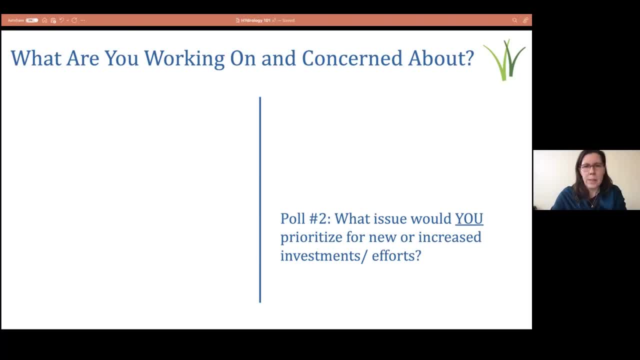 Why don't we give it about 15 more seconds, Chris? Okay, So lots of work on phosphorus, a little bit of work on groundwater and nitrates and a little bit of work on flood risks and damages. Let's go ahead and run the second poll. 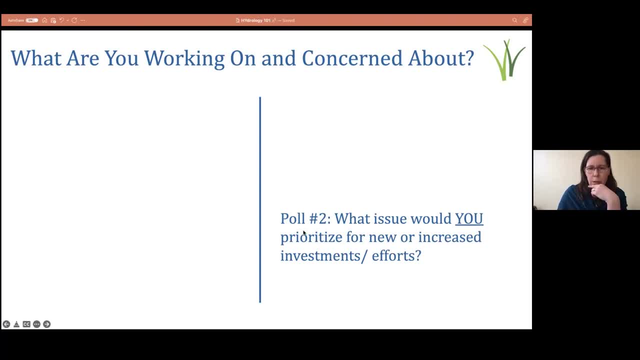 Stop sharing. Here we go. So if you were in charge- Oh, people have already. Oops, there we go. If you were in charge, what issue would you prioritize? And please think about this in terms of not replacing the work you're currently doing, but what would you add or where might you realign, or 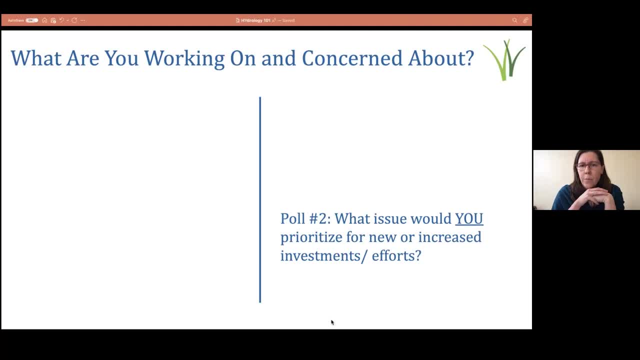 increase investments. Alright, We're close. Run the poll. This is. this is interesting. There's a little more, little more diversity in responses. I can't get to the chat button because the poll sheet is in the way. Come on, Chris. 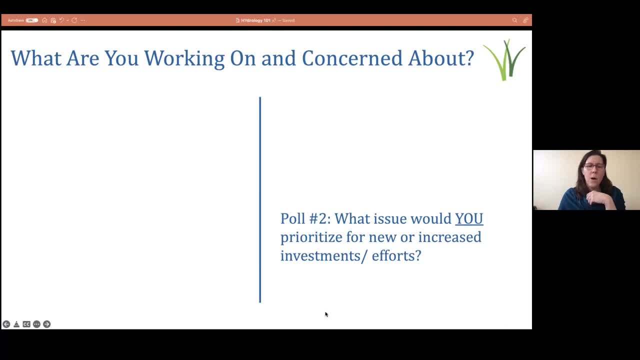 Okay, great way. Any suggestions? Oh yeah, thanks for pointing that out. That's a great point. Why don't you just wait until the polls close and then add your chat response with a indicator of whether you're answering poll one or poll two? if you'd be willing to do that- And I think you can click on the- 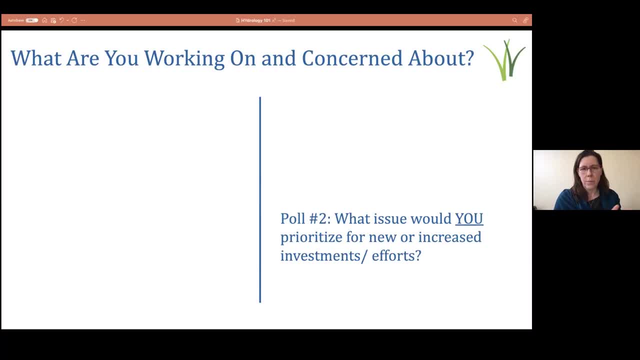 poll question and drag it out of the way. Okay, got it, Chris. it looks like we've kind of slowed down here, So why don't we give this another few seconds? And here we go. So nitrate concentrations: reducing groundwater nitrate concentrations is the slight winner, but still. 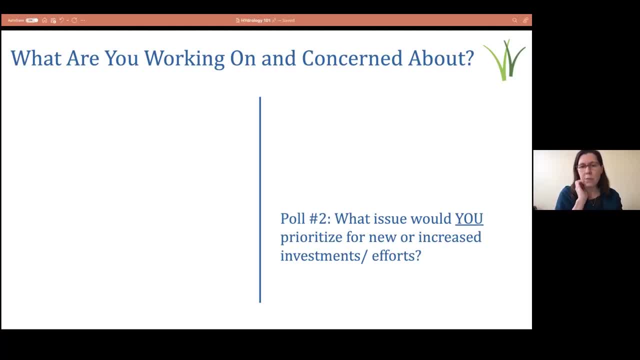 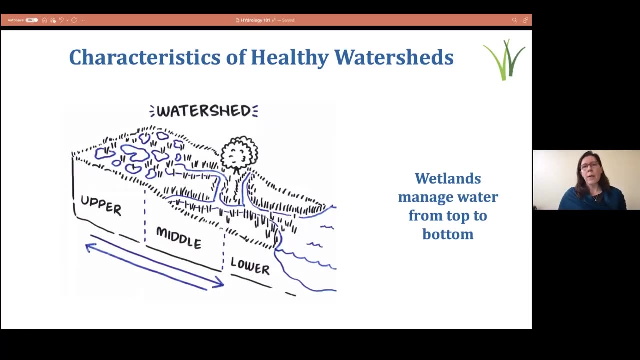 a great deal of interest in phosphorus and maybe a little more interest in flood risks and damages, So I'm going to go ahead and close this poll, And okay. So I'm going to start by talking a little bit about the characteristics of healthy watersheds. 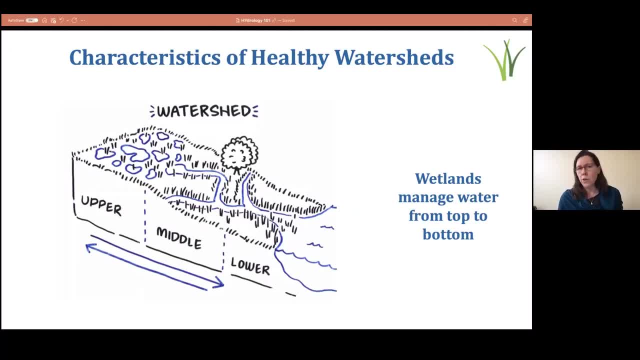 And this probably goes without saying. but we focus on watersheds because all waters are connected And, of course, water flows downhill. So when we're thinking about wetlands and watersheds, we want to keep in mind that wetlands help manage water from the top of the watershed. 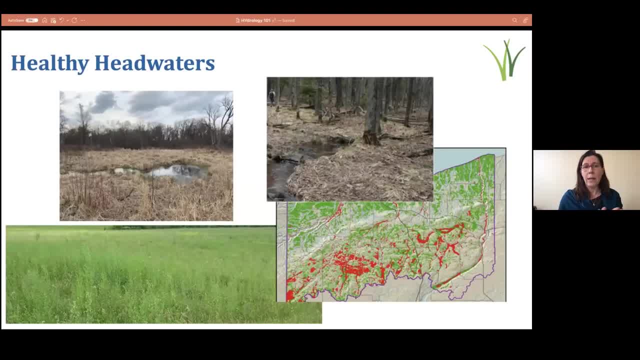 all the way down. So let's talk a little bit about what that looks like. In a healthy watershed, we're likely to have a lot of headwater, wetlands and headwater streams, and there's different kinds and they do different things. 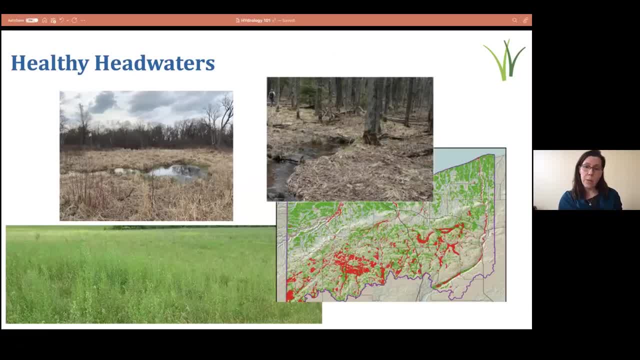 Forests, but a few. a few characteristics that are worth mentioning is they tend to be abundant. It can be wetlands in the form of springs or seeps, or these depressional, ephemeral wetlands that are not connected directly to surface waters but capture rain and snow melt. It can also be the 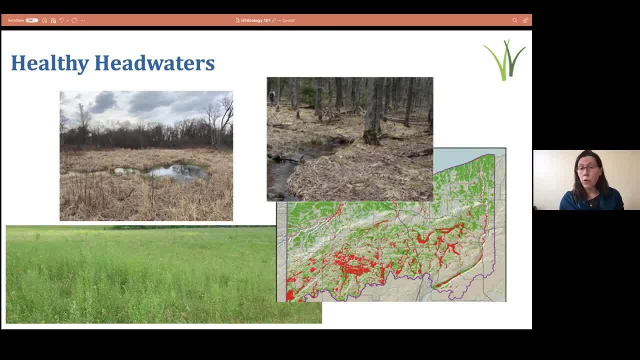 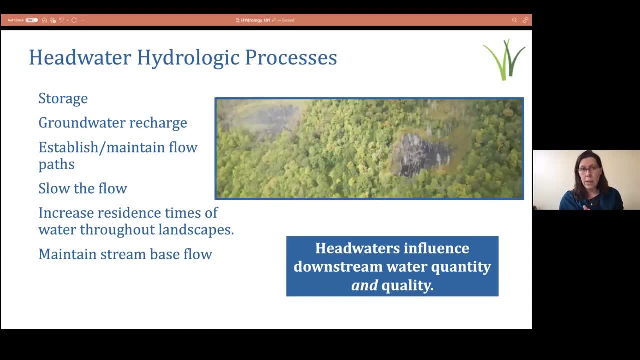 start of our tributaries. Headwaters can occur in agricultural, forested and even urban landscapes, And across the board. they do a lot of things For us, and I'm going to use the word processes a lot in this talk. So the processes that headwater. 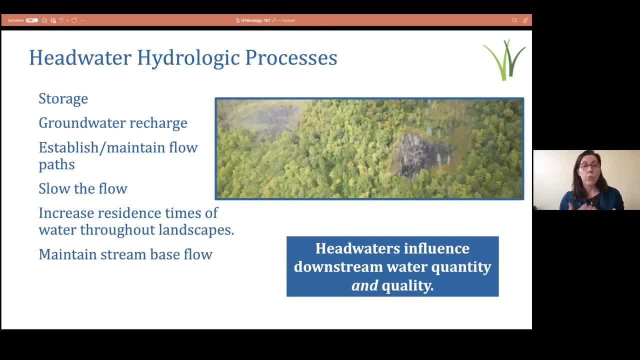 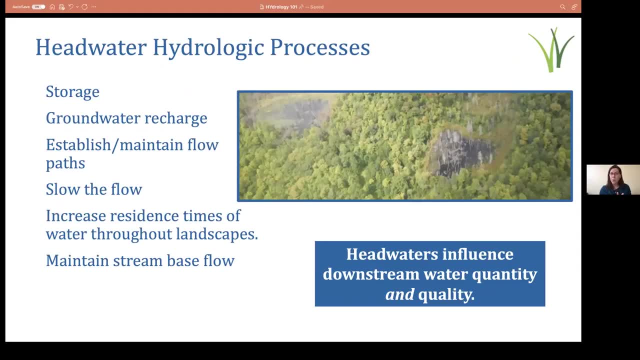 headwaters provide for us are storage, recharge, helping establish and maintain flow paths, slowing the flow, of course, increasing the residence time of the water, so keeping it where it lands, and maintaining our stream base flow. So you put all these together in aggregate across: 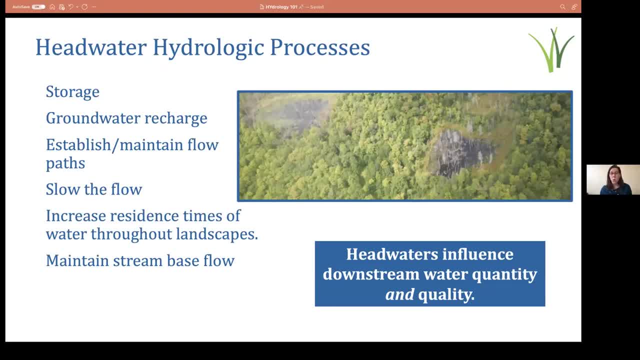 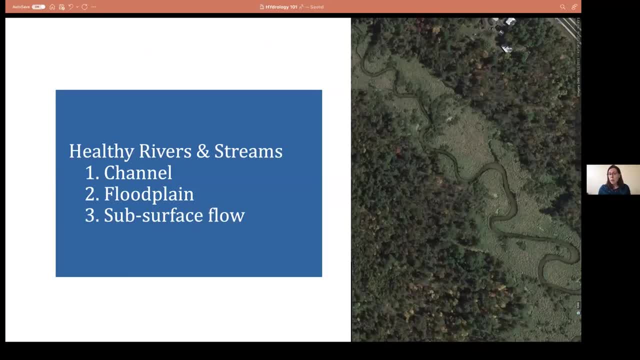 the landscape and headwaters really influence downstream water quantity and quality. Healthy rivers and streams are another very important component of our hydrologic systems, And a river or a stream really has three components. We have the channel itself, the adjacent floodplain and then a lot of subsurface flow, And it's really all three. 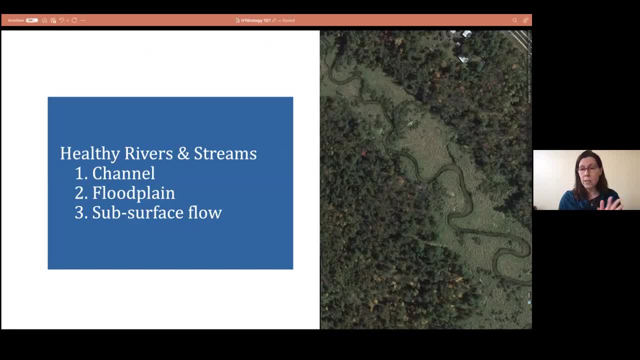 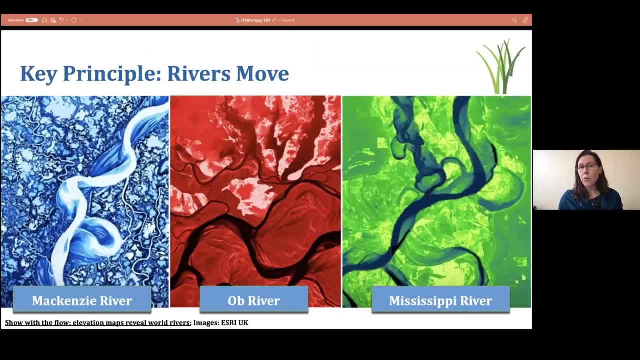 of these things together that constitute the river system and need to be looked at in terms of the health of the system. So I want to talk a bit about some key river principles. The first- and it's a very important one- is the river system, And it's a very important one- is the river system. 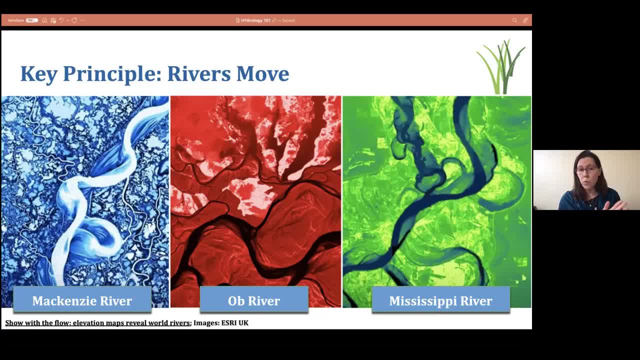 One in the context of how we manage our riverscapes is that rivers move. These are infrared images from a variety of places and some bigger rivers, but you can really see the meander of the channels and the legacy of where that channel moved over time. This is important. 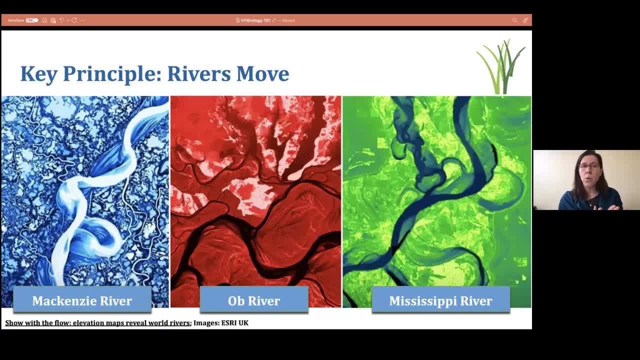 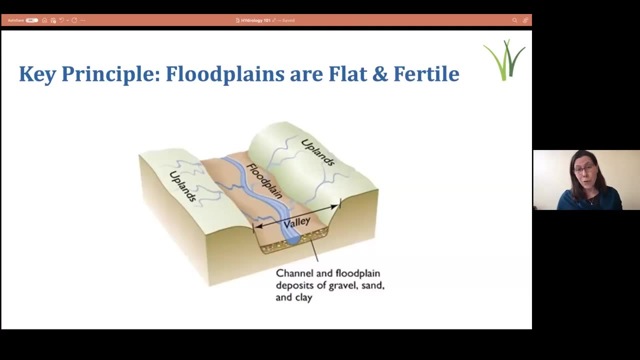 in the context of things like channelization or armoring of banks, where the river might want to move, but we're doing things that are trying to combine it into one specific place or condition. Floodplains are flat and fertile. This is a function of how floodplains form. The river is. 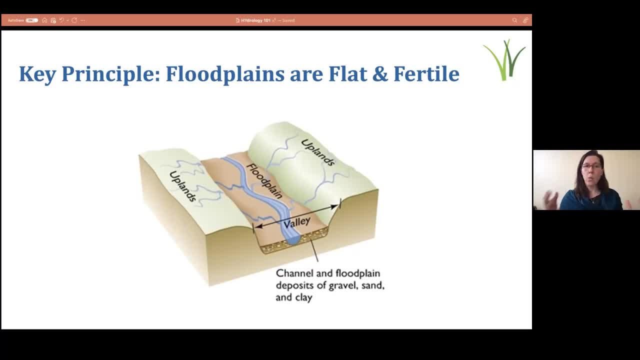 going to naturally cut away at its banks and try to reach an equilibrium where it can rise out and spread across the water in a flat way And, of course, in the process it's depositing materials, sediment and other things that are decomposing and adding. 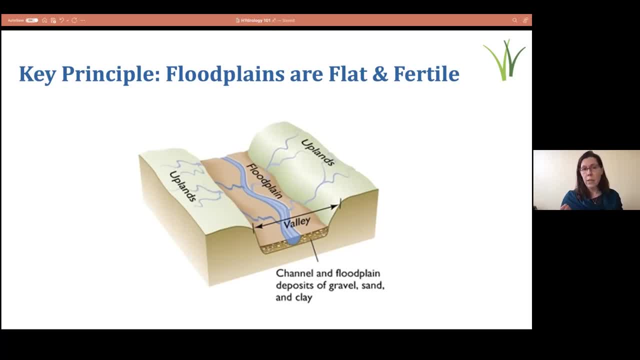 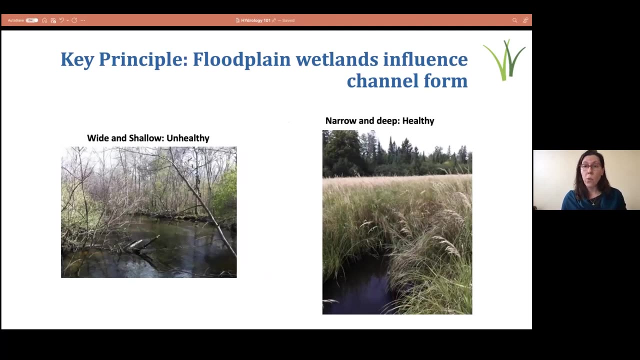 organic matter and other chemical constituents- positive chemical constituents to that floodplain. So flat and fertile is what we're going for when we have a healthy floodplain. Also important is that floodplain wetlands influence the channel form I'm talking about. 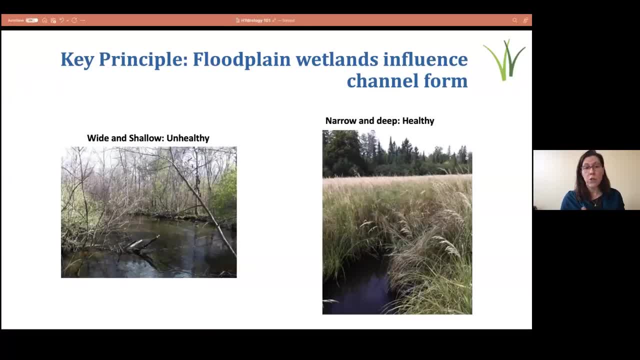 both the physical condition of the channel and the processes. So these pictures here show an example of an unhealthy stream. It's wide, It's ankle deep, It's kind of choked with brushy material, vegetative communities that have root systems that don't hold the banks very well. Versus on the right, we have a really nice. 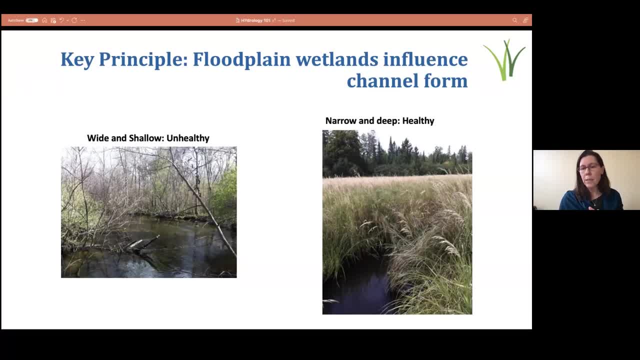 wetland floodplain connected to the stream. We have a narrow and deep channel with nice overhanging banks, very stable, cold water, good fishery conditions, et cetera. And another thing to remember, even though it's not always pretty, is that messy can be good. 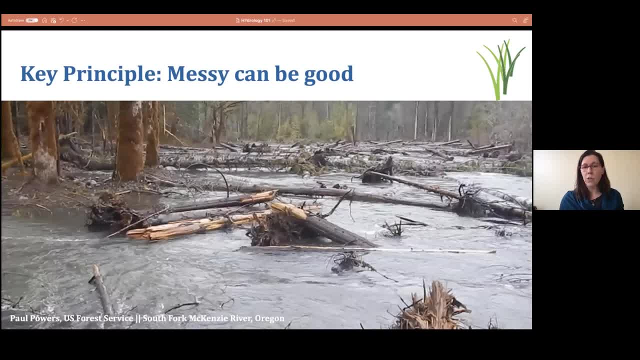 When we have woody debris in our systems, we have a lot of things our systems are not going to have. The river system needs friction, habitat, micro refugia, nutrient inputs, et cetera. So maybe not the best thing for casting a line, but sometimes very positive and healthy for 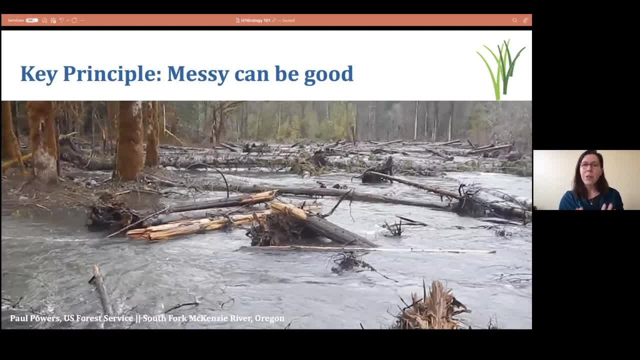 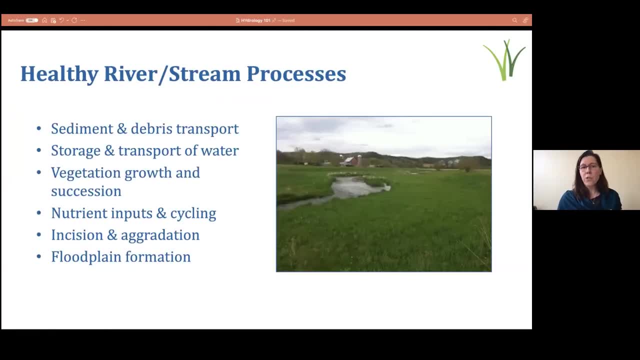 the river system itself. So messy isn't always bad, unless you want to not hook your line. So, when it comes to river and stream processes, I've mentioned a lot of these already, but we've got sediment and debris, transport, storage and 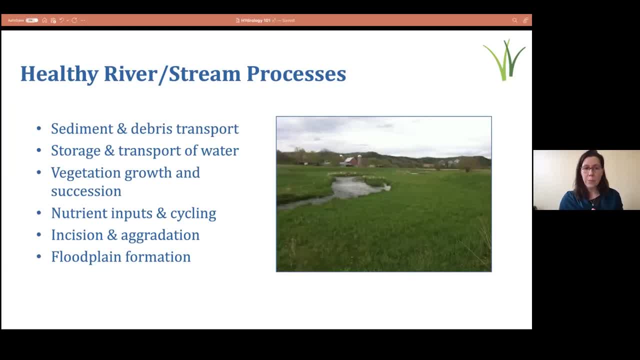 transport of water, vegetative growth and succession, nutrient inputs and cycling. So nutrients come in, nutrients go out. incision and aggradation as a normal, healthy process. rivers change laterally, longitudinally up and down and healthy floodplain formation. 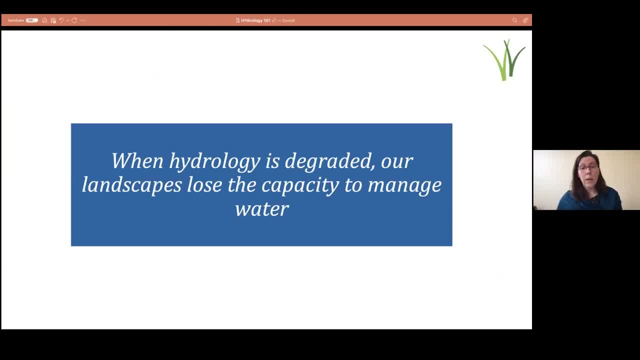 So, when hydrology is degraded, our landscapes lose the capacity to manage water. Let's talk about a little bit, and some of these will be obvious, but I want to go through them because I want to think about them a little bit. So let's start with the first one. So, 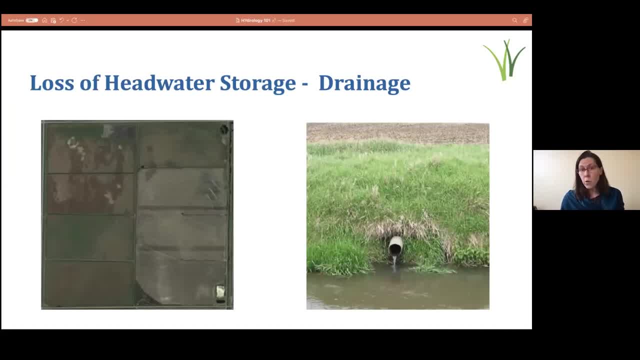 we're going to talk about them in aggregate. So loss of headwater storage: One of the ways we've removed a lot of our headwater storage and runoff management capacity from our landscapes is through drainage, whether that's ditching or tiles in agricultural and urban settings. 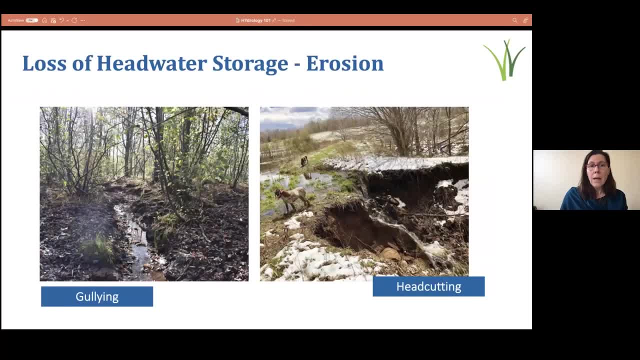 It's very widespread in Wisconsin, But we also lose a lot of headwater storage through erosion. So these are pictures of gullies and head cuts that are happening in ways that are cutting through wetlands that normally would be providing a lot of storage, And you can see in the picture on 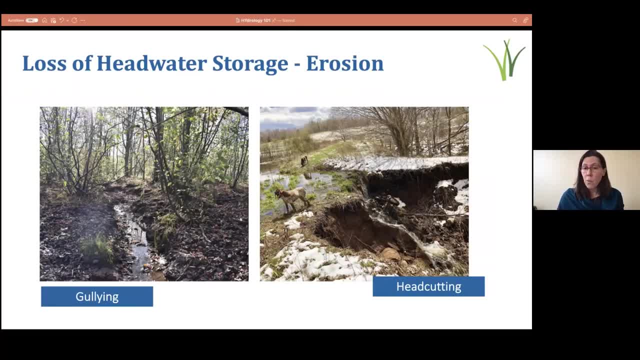 the right. it's a real gusher right. There's a lot of water draining out of that wetland and a lot of soil moving in the process, So really unhealthy conditions that are contributing to our runoff management problems And this kind of non-channel. 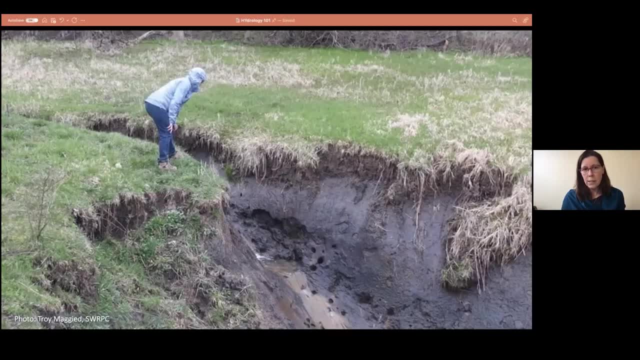 big-scale erosion is common across the state, particularly in our steeper landscapes. This is an image of an area head cutting downstream from a development project that's up on a hill above a wetland, And, of course, what you can't see in the photo is it gets a lot worse as you. 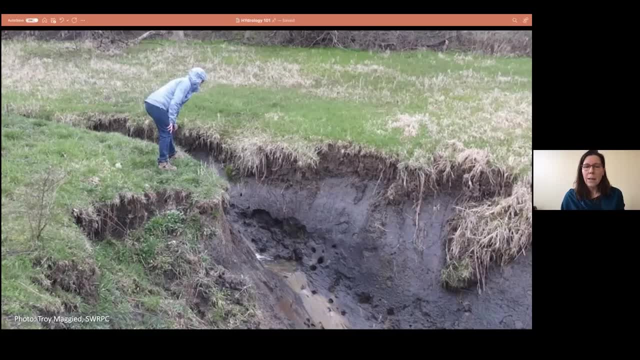 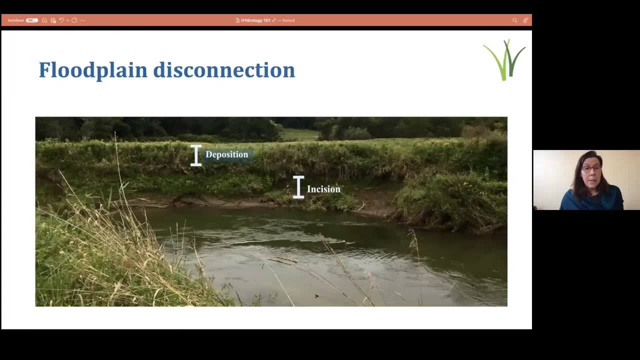 go downstream And we're seeing a lot of water and material eventually making its way to our river systems. Floodplain disconnection is another very, very common indicator of poor stream health in Wisconsin. So floodplain disconnection is another very, very common indicator of poor stream health in. 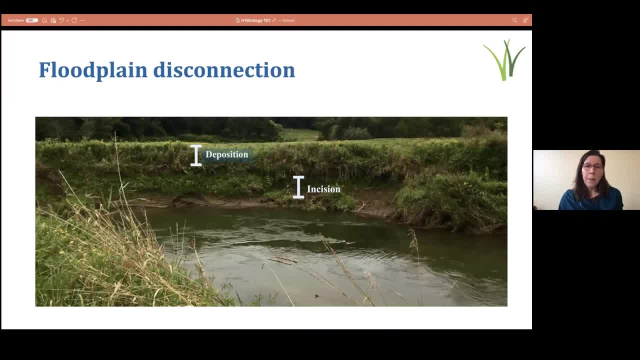 Wisconsin. So floodplain disconnection is another very, very common indicator of poor stream health in Wisconsin. In this slide you've got deposition, which probably came first. This is, you know, historic, an artifact of when a lot of the soil moved off of our steeper slopes and deposited. 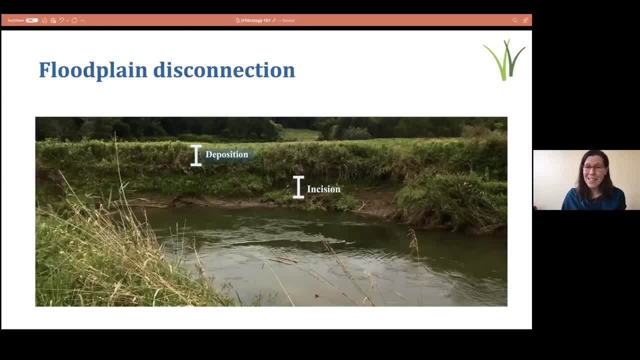 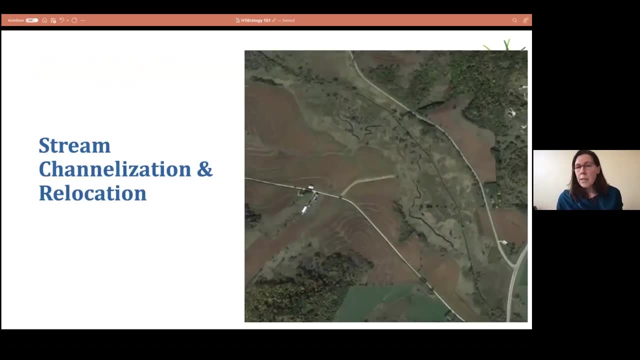 themselves on top of our wetlands And then also incision where uncontrolled flows are cutting down the bed of the stream. In this case, both are at play in this picture- And stream channelization. So this is a photo of Fancy Creek in the Driftless area And you can see 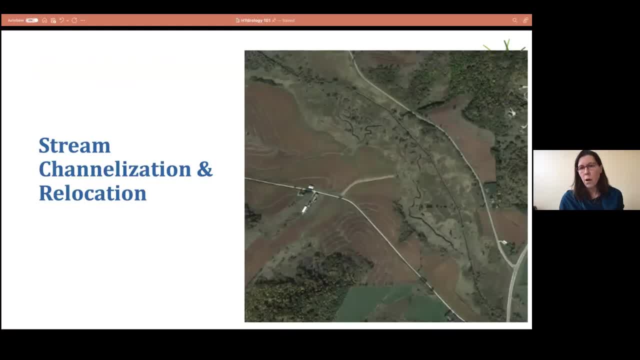 both the current channel, which is, you know, long and straight and pushed to the side, versus the former channel, which was meandering, which would have allowed slow movement of water, And you've got a nice wide former floodplain here And I'll show you a picture in a few moments of what this 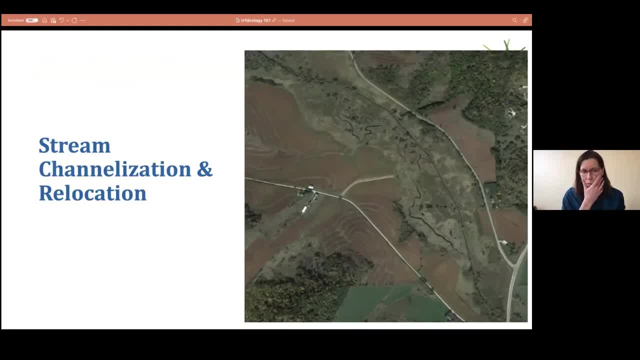 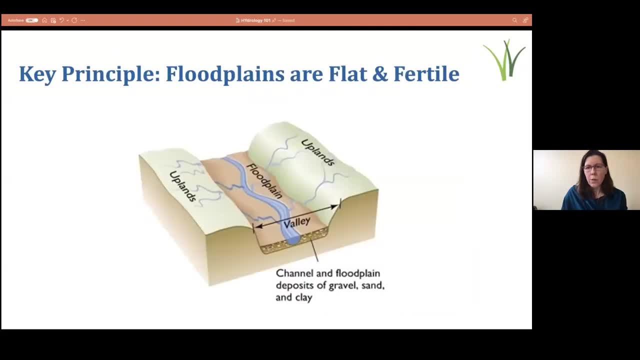 system looks like today, And you know one of the things that I think we forget because we have so few stream systems that are healthy. I'm going to go back real quick to this picture. Oh no, I'm not going to do it because it's going to go back too far. 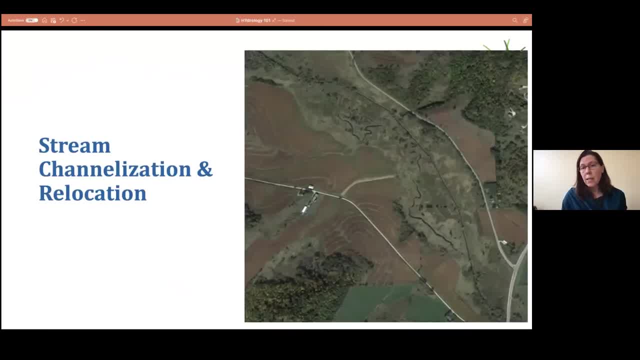 You know, we used to have a lot of rivers and streams that looked like this: A nice slow meandering channel connected to a very robust and big sedge meadow floodplain, And we have so few of them now that we've almost forgotten that that's what our river systems. 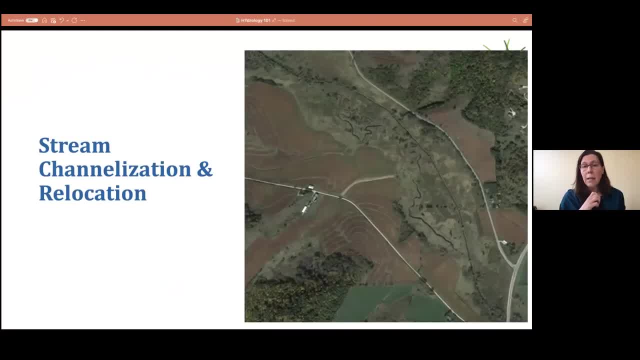 are supposed to look like. Sometimes the channel would get lost altogether in the wetland meadow because it would just sort of the river would sort of disperse and then come back together. So we don't see that much anymore. but we have a lot of opportunities to restore those conditions. 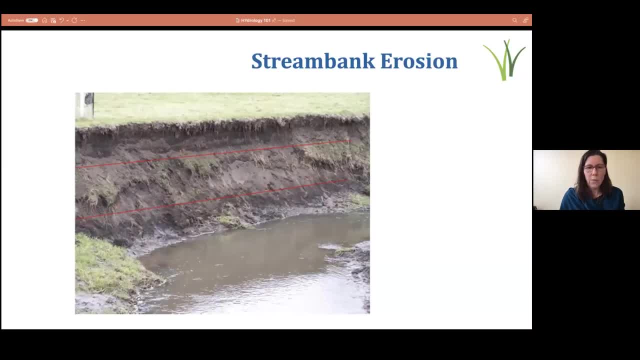 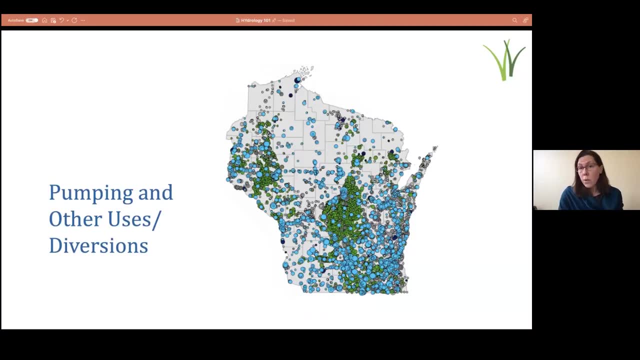 And, of course, stream bank erosion very common. You all have rivers and streams that look like this in your communities. Obviously, there's a lot of other ways that we've altered hydrology. This is a picture that you all have seen of high capacity wells across the state And 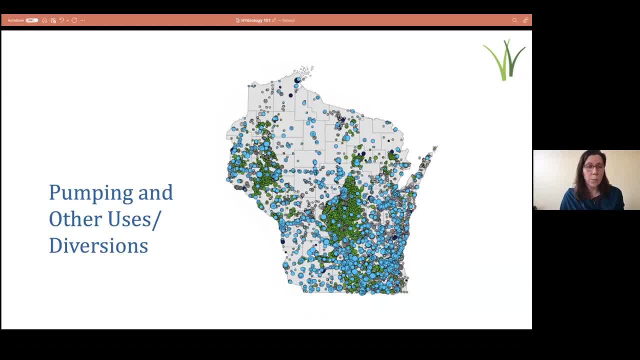 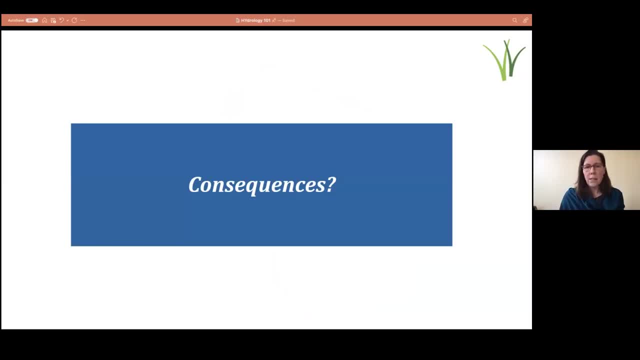 there's other ways that we're using and diverting waters from our streams, our streams of water. So this kind of large scale hydrologic alteration obviously has consequences that you're all familiar with When our creeks look like this. now, this is Fancy Creek, This is that picture. 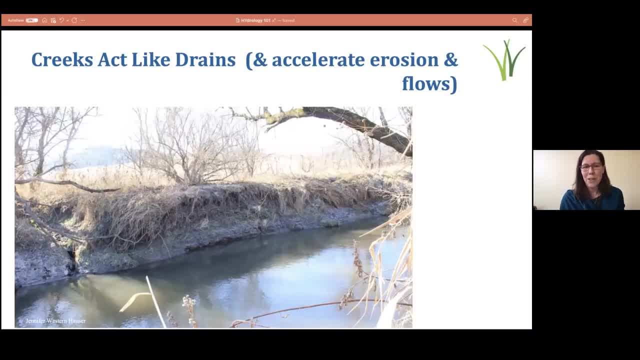 that I showed of the aerial photo with the remnant meandering stream and the current channel, straight long channel. Our creeks are acting like drains right, Just like that upper watershed. loss of storage. We're accelerating erosion and flows and moving a lot more water and a lot more material. 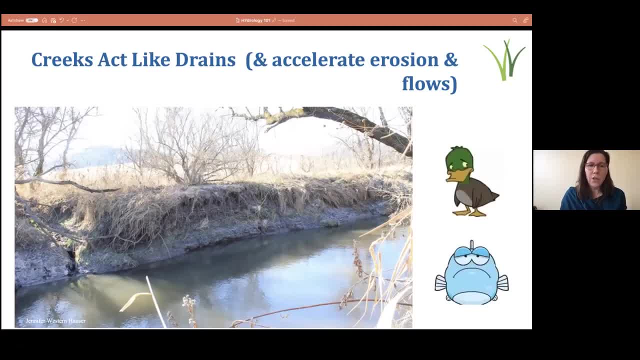 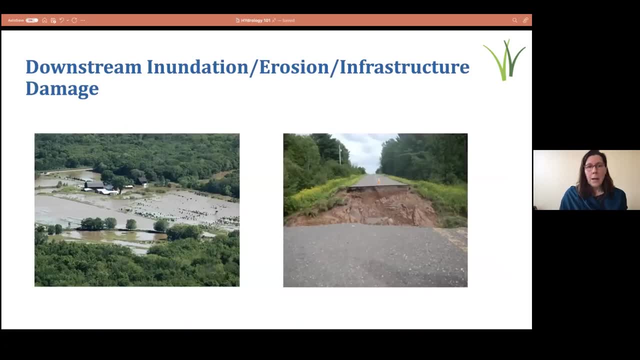 downstream And of course, it's not great for the fish and the wildlife, Although, ironically, in this channel there are still a lot of trout. All of this loss of storage results in downstream inundation and erosion, And the combination of the two is causing a lot of infrastructure damage in. 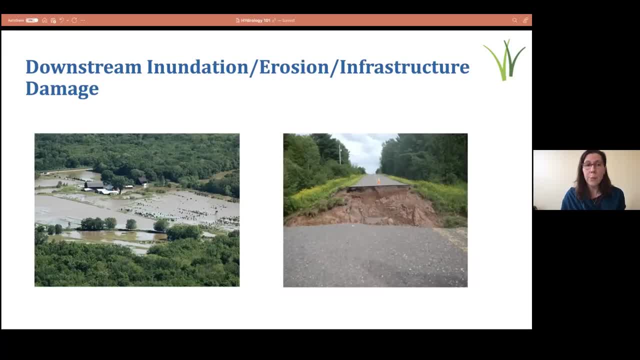 a lot of communities. You'll hear more about that in the next session. but particularly covert blowouts is a major problem in a lot of communities and a major headache for a lot of our counties and towns, And muddy and eutrophic waters very familiar to all of you, I'm sure. 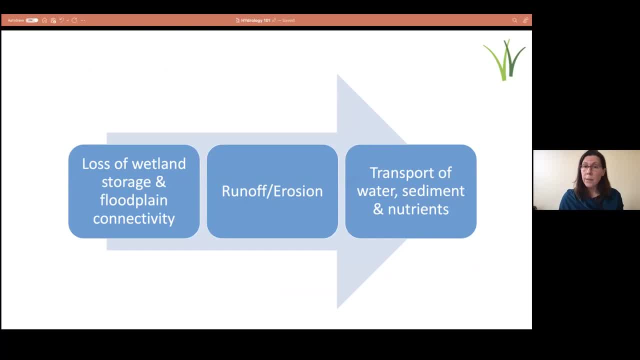 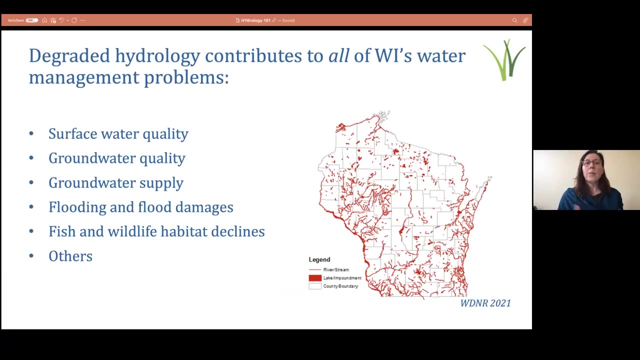 So, when we think about this from a process perspective, we're talking about loss of wetland storage, loss of floodplain connectivity leading to unnatural levels of runoff and erosion or problematic levels, and the transport of water, sediment and nutrients downstream. The message I want to share here, then, is that you know we have a lot of degraded 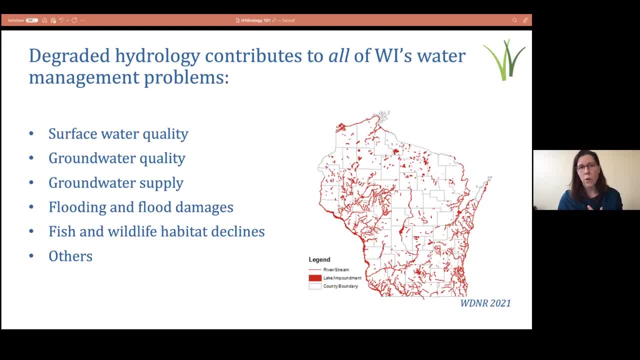 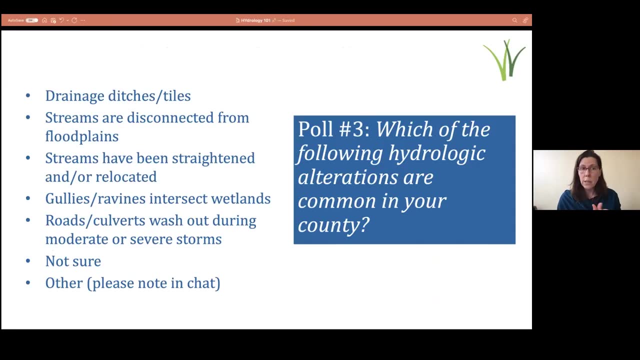 hydrology in Wisconsin And it is contributing to all of our water management problems, whether that's surface or groundwater, quality, groundwater supply, flooding, fish and wildlife habitat declines, etc. So let's stop and take another poll to get a feel for what you're seeing in your communities. 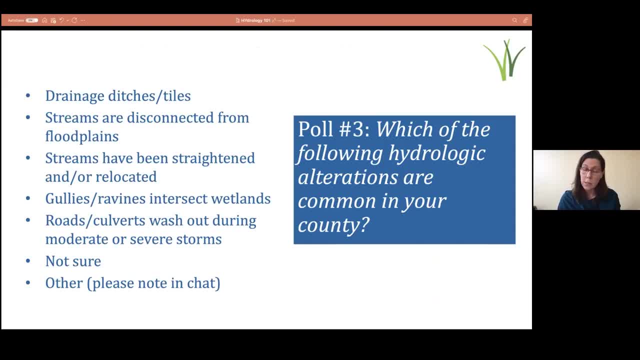 The question is which of the following hydrologic alterations or consequences therein, are common in your county. So this is poll number three, Chris, And thanks to all of you for being so engaged. It's nice to see responses in the 100 and 125 level. 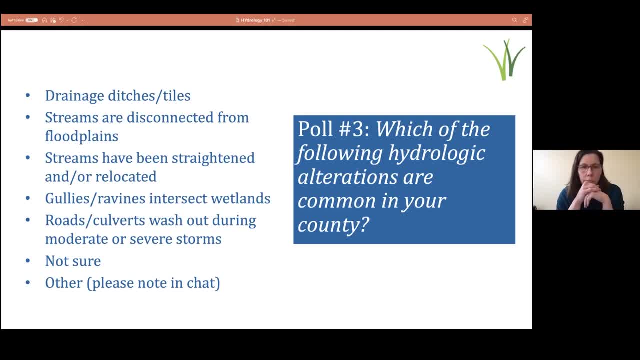 And if it's not apparent, this isplease you know, choose all the others. And if it's not apparent, this isplease you know, choose all the others. 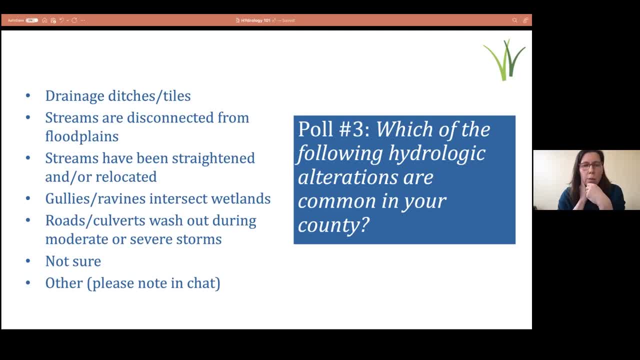 which is, you know, we briefly mentioned, apply. So no one, no one, unfortunately, no one right answer. So lots of ditching. 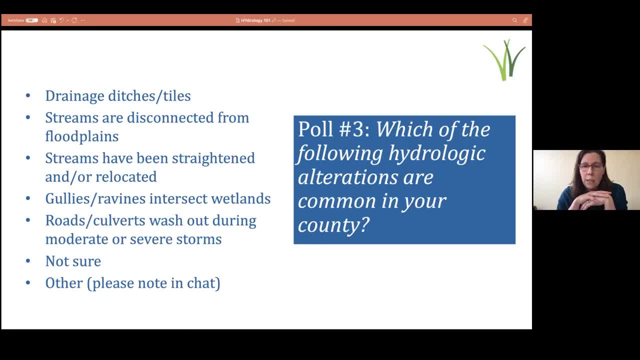 lots of flooding, lots of plain disconnection, lots of channelization, Gullies, ravines, road, culvert, washouts- Not too many, not sure, And I'm actually glad to see that. It means that you know. 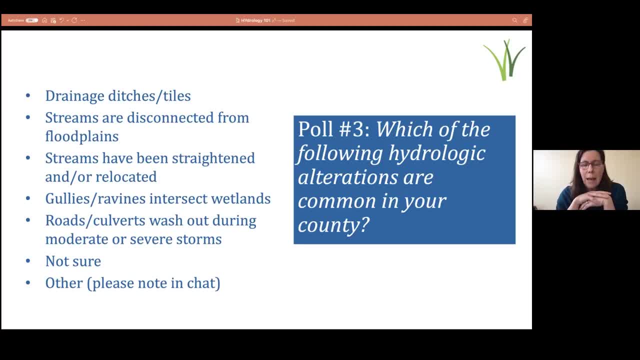 folks are at least pretty familiar with this aspect of hydrologic alteration in their communities. It's kind of hard to ignore some of it. Okay, I think we'll probably slow down enough that we can end the poll, and I'm going to. I'm going to pull the results off my screen here. 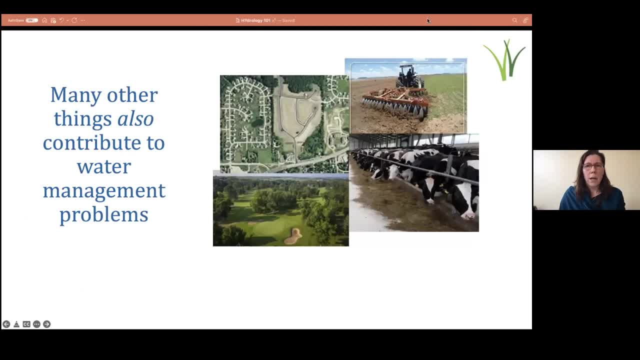 Okay, So to be clear, a lot of other things- I understand many other things- also contribute to these water management challenges and problems. right, And we don't necessarily need to go into that. What I will say is that some of these other stressors- 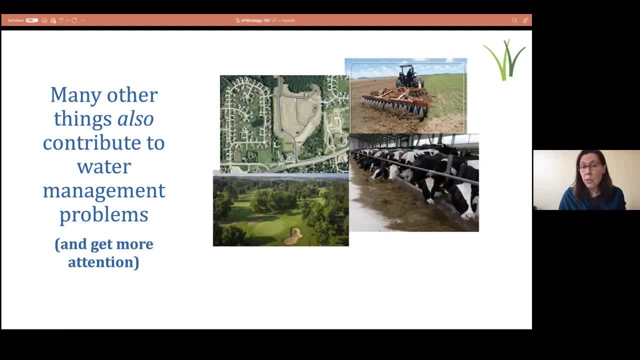 tend to get a little more of the attention and the interventions that we're employing, And the thing that we need to be thinking about is: you know, there's really no one cause to all of our water management problems, And because of that, 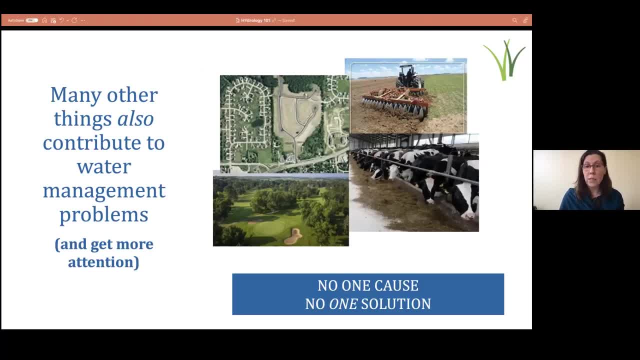 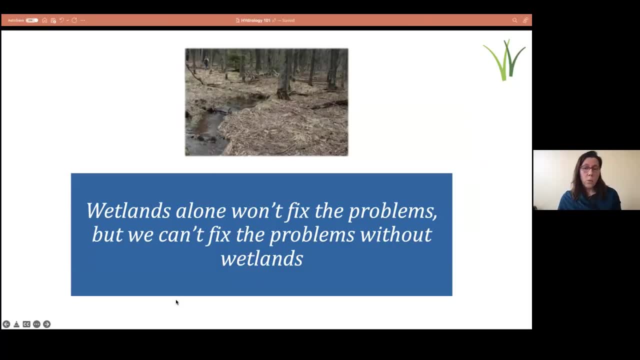 there's no one solution. We need a lot of different tools to address these problems because they come from a lot of different, different causes. So we like to say wetlands alone won't fix the problems, but we can't fix the problems without wetlands. 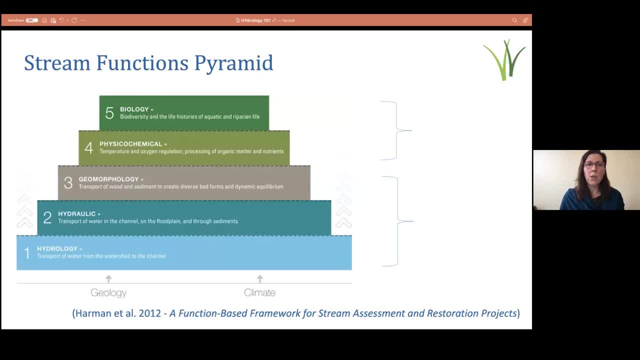 And I'll hopefully make that abundantly clear throughout the course of this talk. So so I want to talk about this in the context of of this extreme functions pyramid, which was put out in about 2012.. In Wisconsin, we spent a lot of our efforts investing in 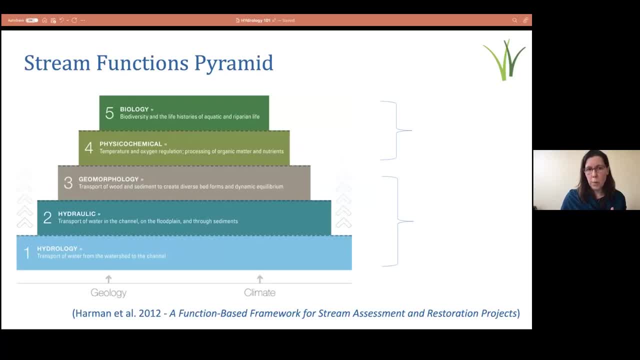 interventions that are designed to deal with problems at the top of this pyramid: the biology or the physical, chemical attributes of our streams and wetlands, And I'll use- I'll use wetland restoration as an example. I'll pick on wetlands first. 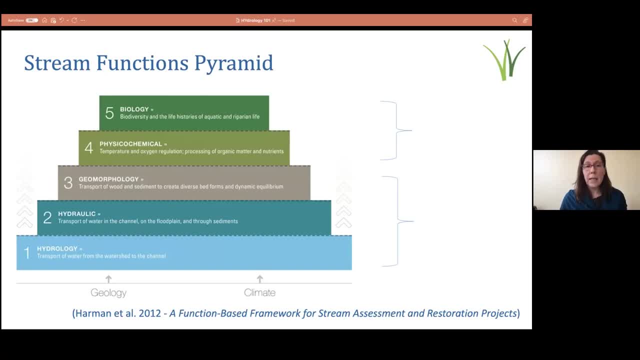 We've we've been very focused historically over a decade, decades and decades on wetlands for wildlife And a lot of the restoration that has happened in the name of, of of wetland improvement, has been wetland enhancement with the purpose of. 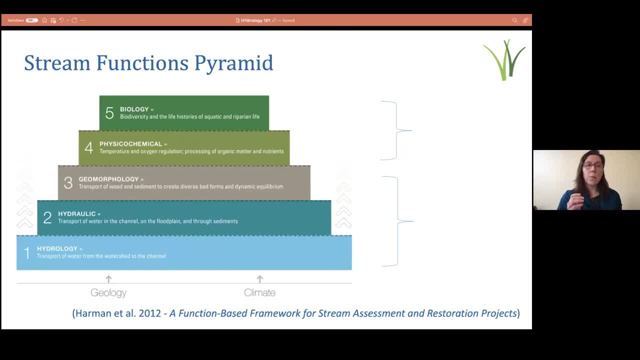 improving the vegetative community to provide more adequate cover, nesting cover, or or, or forage, or whatnot, And, and those things are really important, right, And the same might be. you could also use the example of, you know, buffers. 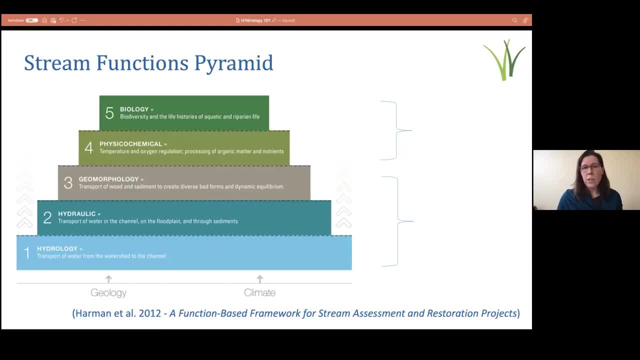 where we're looking to sort of treat runoff before it reaches our stream. But here's the thing. what, what we know from the science, from a hydrology science, is that it's the bottom three tiers of this pyramid: the hydrology, the hydraulics. 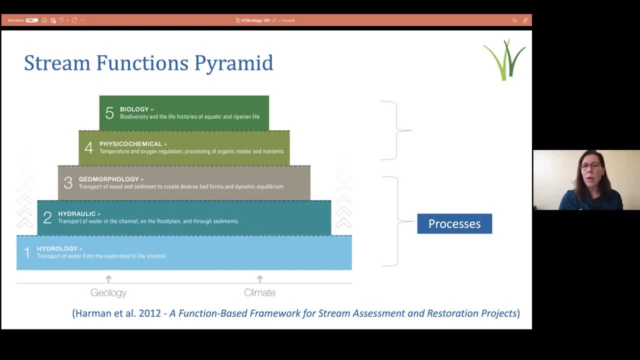 the geomorphology. Those are all just fancy words to describe how water moves, what's in it and what that water movement and other processes are doing. These are: these are the processes that, when they are healthy, support the responses in the system, which is the chemistry. 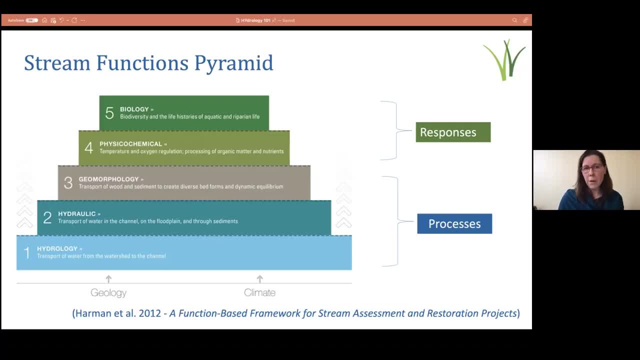 the biology, the habitat, the water quality, et cetera. So the idea here is that if we have healthy processes, we set the stage for the conditions that are necessary to have the stream and lake attributes, or the to achieve or to more. 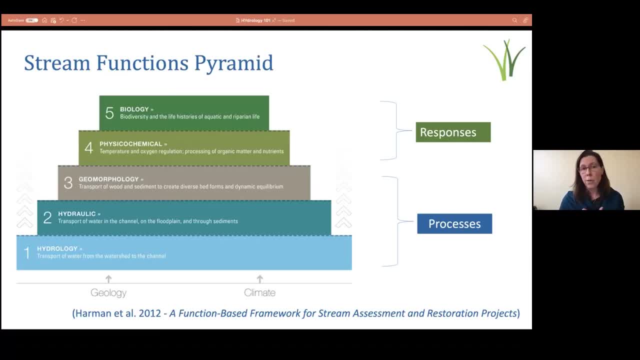 likely achieve the indicators of aquatic resource health that we're measuring or or watching. Okay, Hope that makes sense, And I think Megan's going to pop a link to this stream pyramid in the chat. There's a version of it that has a little more detail in. 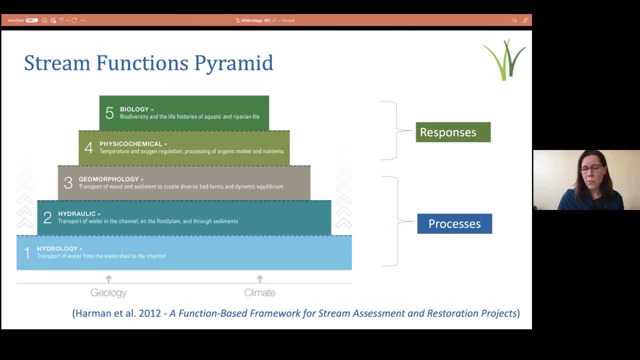 terms of what the parameters are for each of these five tiers. So you know, I'm going to leave the slide there actually for a moment, And I think, Megan, we could look at the chat and take a couple of questions here, just to break up our time. 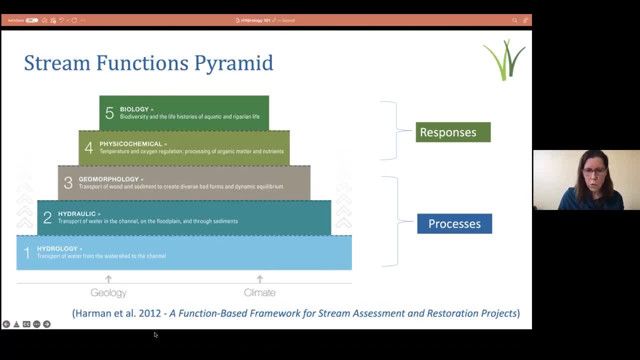 I have trouble seeing the chat, So why don't you unmute and tell me if you have specific questions that we need to you know answer? So there's one question right now. Current egg performance standards- NR151- allow for cattle to have access to surface water. 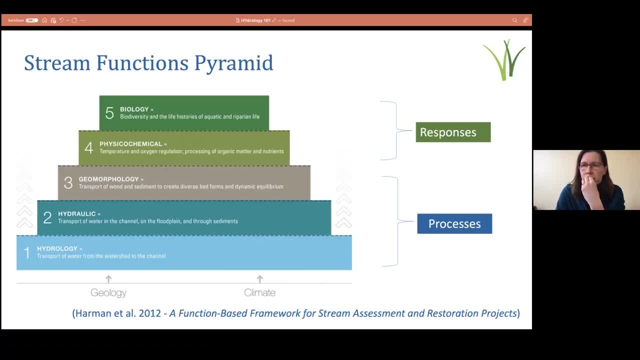 as long as vegetation is maintained on the bank's flash floor line. Can you describe the impact cattle have in wetlands? The rules may not prohibit grazing or pasturing of wetlands, but what would be recommendations if a landowner was to do such? 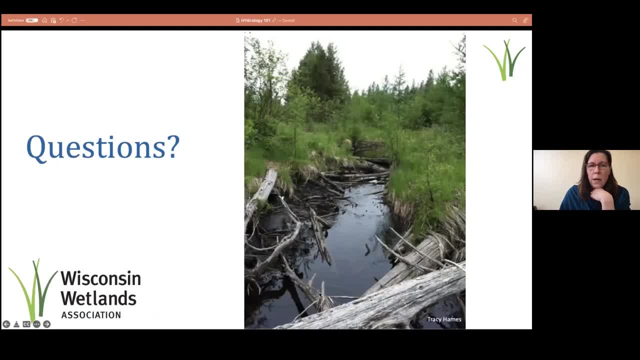 Yeah, that's a great question. Yeah, that's a great question, Thank you. The answer is always: it depends, but the grazing can actually be a really effective wetland management practice. It's not necessarily a terrible. it's not only not necessarily a terrible thing. 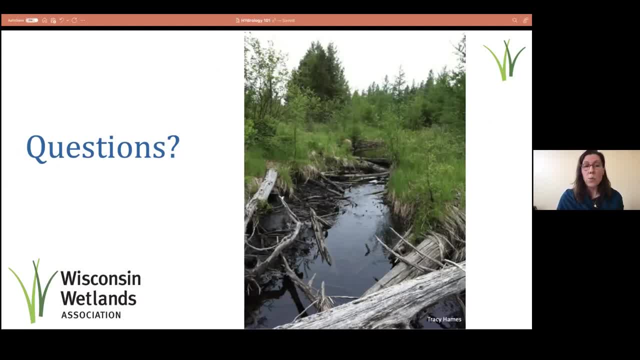 sometimes it's a necessary thing because it's regenerative right And so, but it's always about the right, you know, the right amount of cattle and the right amount of pressure. So we'd actually like to see wetlands. 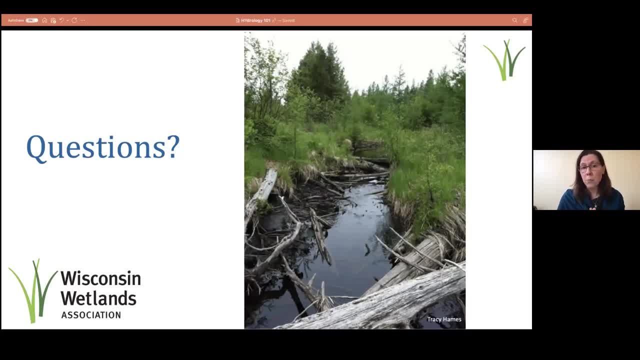 We'd like to like to see grazing as a planned management practice more frequently in a lot of our wetland systems, because it's a it's a good way to help manage some of the invasive plants and get back to a more diverse and healthy wetland plant community. 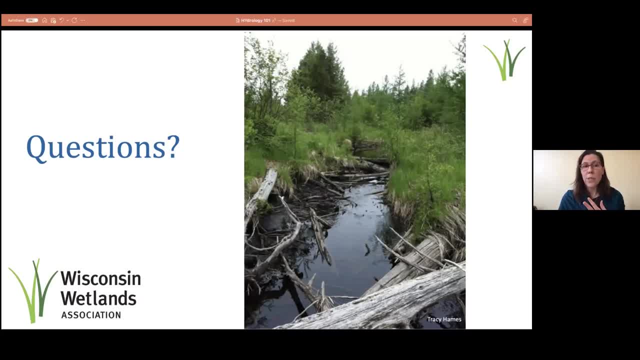 It's not appropriate for every site right, And so this is where having some support to make those decisions about where it's appropriate and where it's not is really beneficial. It's a big topic. The next one, The next one is just a statement. 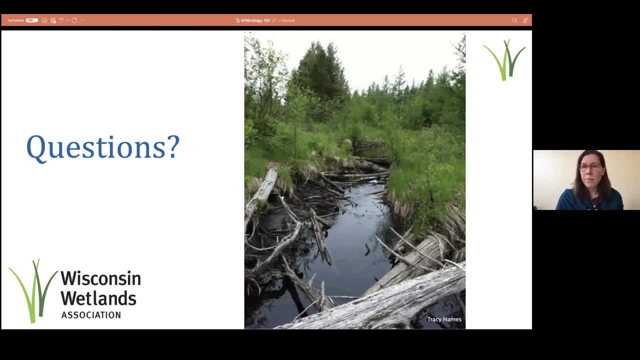 not necessarily a question. So what you're saying is we are treating the symptoms rather than the disease, Exactly. And then one more question: There's a lot of focus on improving soil health to increase weight. Sorry, excuse me. There's a lot of focus on improving soil health to increase rainwater infiltration. 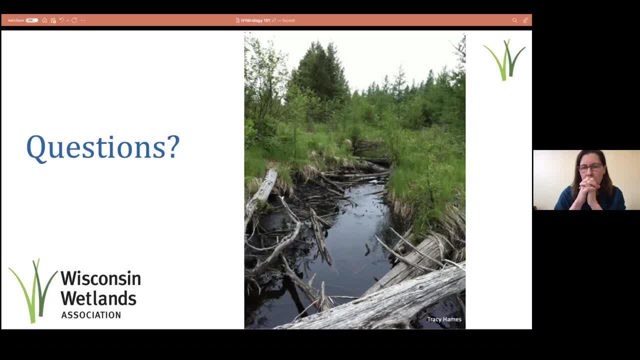 How much of an impact will that actually have on the flashiness of runoff events? I can have a lot. It can have a lot of impact because what we're talking about is storing and holding the water where it lands, And you can look at a situation like a drainage ditch or a disconnected floodplain, where 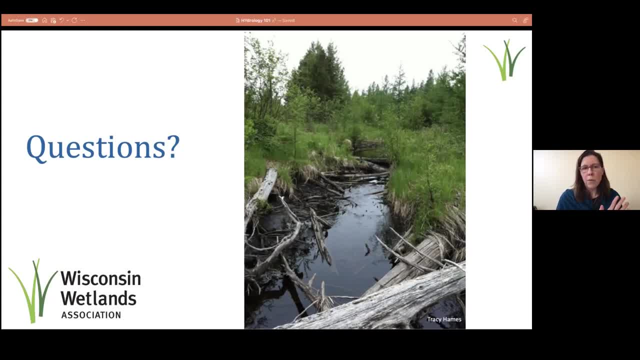 you know that water hits in the spring or following a big rain event and it's gone right, Fire hose right downstream And and the goal of these kinds of practices really is to stop the spread of the disease, right Yeah. 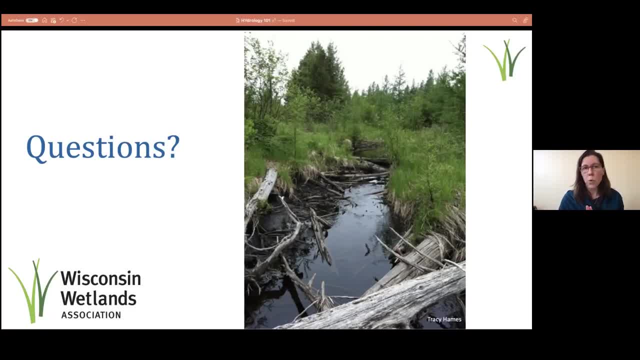 And the goal is to smooth the hydrograph. So instead of having all the water move in a short duration at a high spike, we want to really even out, lower that curve and have that water moving more slowly And then also, of course, available for us at the end, when you know at the end later. 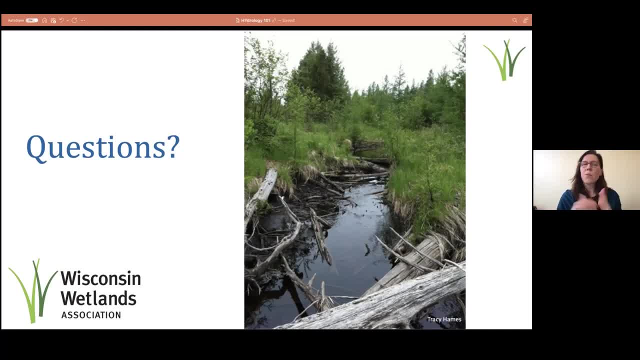 in the season when we need it. And there's, you know, there's modeling and other ways of sort of estimating what those changes in the hydrograph or changes in the during the season make Absolutely. Next question: Duration and frequency and flashiness curves can look like that's not my area of expertise but there's a lot of people in the state that that do that work and understand those processes very well. 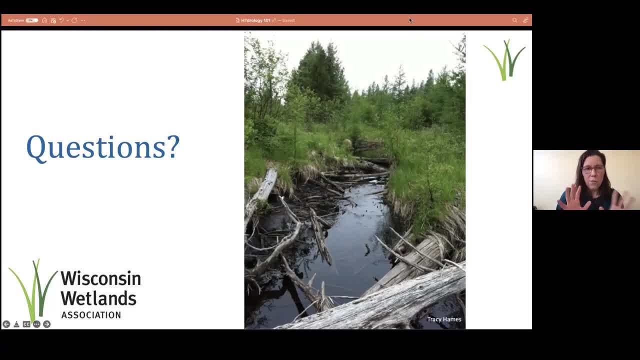 And why don't we? why don't we hold there? and we're going to structure this so we have time for questions at multiple points along the way. so i'm going to move on, but please keep the questions coming in the chat And i'm I wish we were in person and could have more, a better forum for discussion. 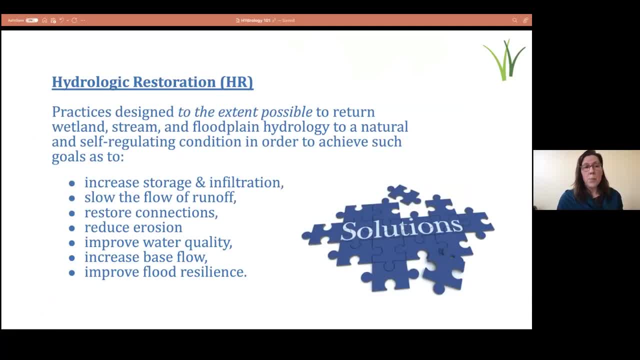 So what are we talking about? how do we get these, these kinds of practices and these kinds of practices- excuse me- processes back on the landscape? Here's our working definition. it's not textbook, it's just the one we use for hydrologic restoration. so practices designed. 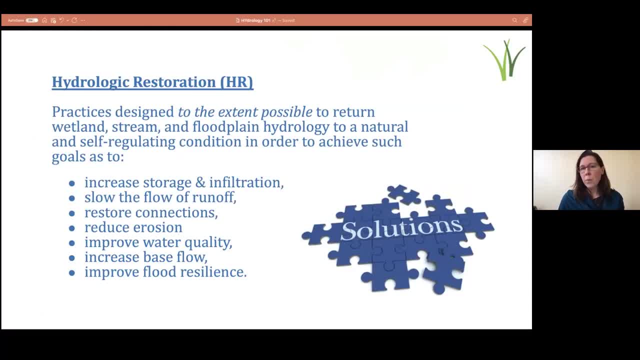 To the extent possible, to return wetland stream and floodplain hydrology to a natural and self regulating condition In order to achieve such goals as to- you know all the ones we've already discussed- storage and infiltration, slowing the flow, restoring connections, reducing erosion, etc. etc. so we're talking about wetlands and floodplains as solutions. 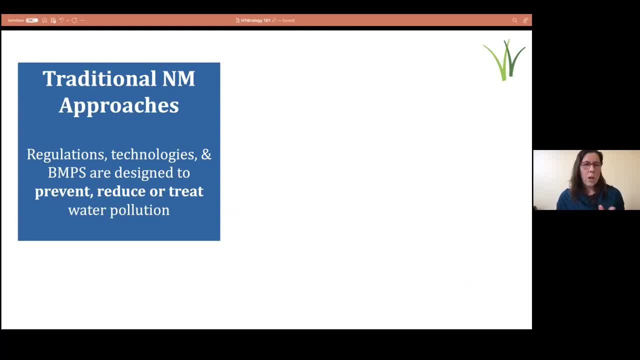 Now, This slide came from a talk I gave to a bunch of policymakers across the Great Lakes region last week. it was a nutrient management talk, so i'll use it as an example, And it makes the point that was just made in the chat. so a lot of our traditional nutrient management approaches, our regulations, our technologies are 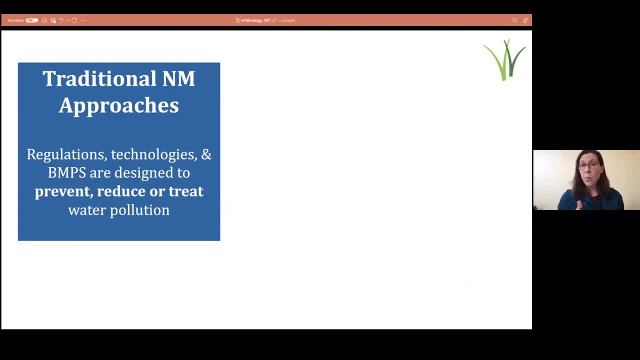 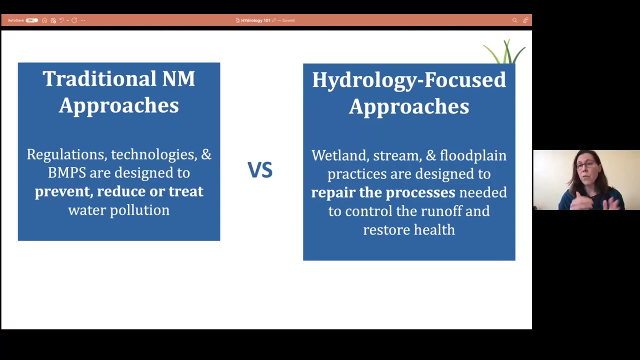 Designed to prevent, reduce or treat pollution right, and this is appropriate. we need these because we have pollution. we have a lot of inputs that are causing problems and a lot of practices that, if not well implemented, can contribute to our nutrient management problems. the difference between these kinds of practices- by and large- not unilaterally, but in general difference between these and hydrology focused approaches- is that our wetland stream and floodplain practices are designed 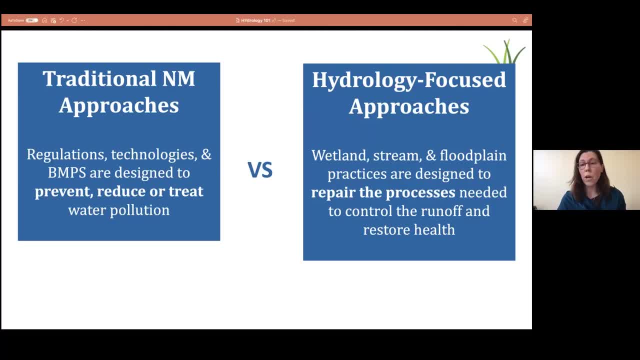 to To repair the processes needed to control the runoff and restore health. so site specific practices to address symptoms versus system level level improvements to address root causes. another way to look at this is Prevent- or Prevent damage or or heal the system right, we need both, we need a lot of both, but i'd say in Wisconsin we're. 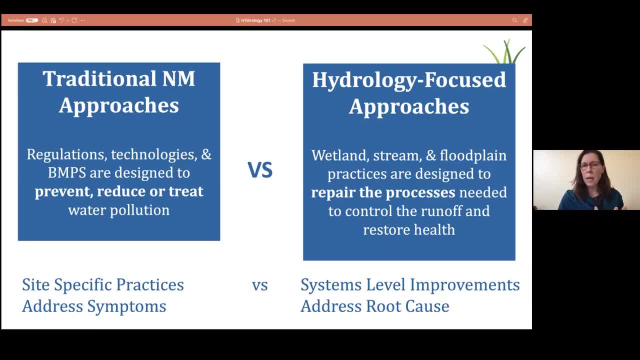 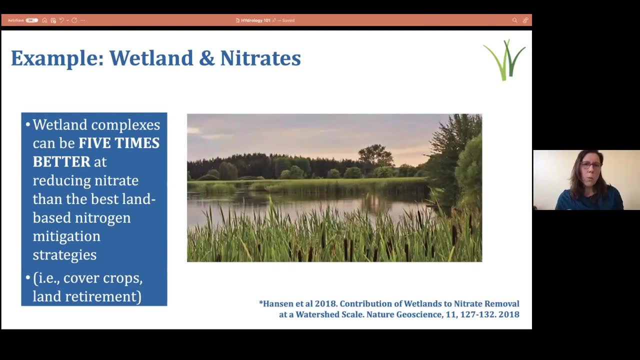 Spending a lot more of our energy and investments on the practices to prevent problems or prevent damage, as opposed to restoring our system and its complexity. here's a good example: we there's research that's come out of Minnesota that's showing that wetland complexes can be five times better at reducing nitrate. 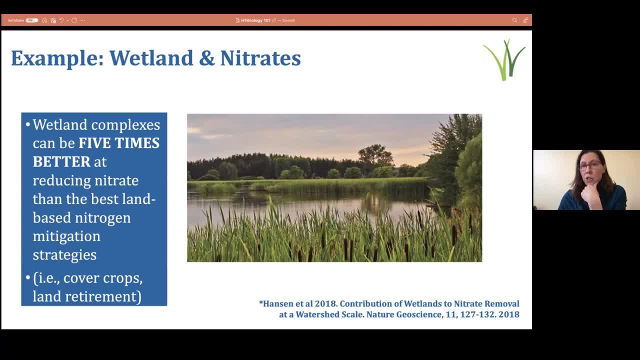 concentrations than the best land based nitrogen mitigation strategies such as lab or crops or traditional land requirement at land retirement. excuse me, I won't get into the biogeochemistry of this, but basically the fact that wetlands are saturated all the time gives us the bacteria that's needed to metabolize my traits to nitrogen. 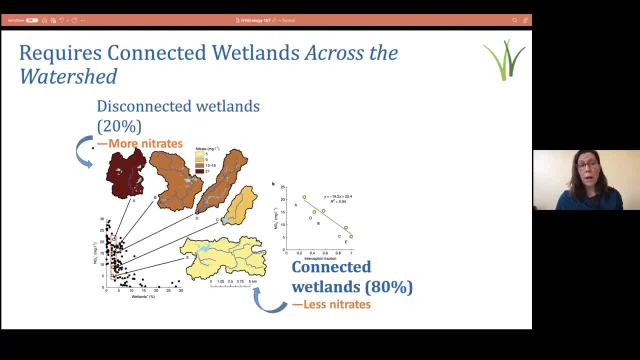 gas. what's important to know about these findings is that it requires connectivity, and this is a fairly complicated graphic, but essentially it just tells us that The more connected our wetlands to the stream network, the better effect it's going to have on nitrogen concentrations in our 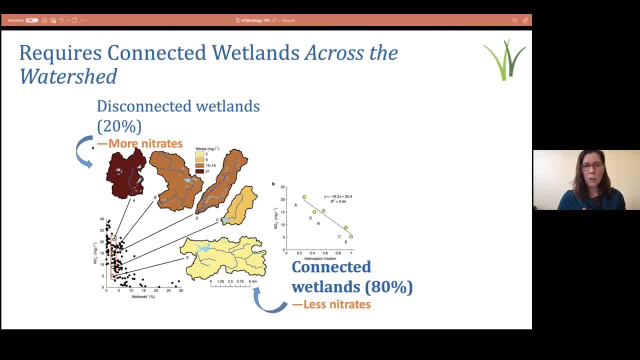 surface waters. That's what this- uh, it was a meta-analysis- looked at. So the the the disconnected wetlands are going to have higher nitrates in the system, The more connected wetlands are lower. So this tells us. when we think about opportunities, so say we want to be. 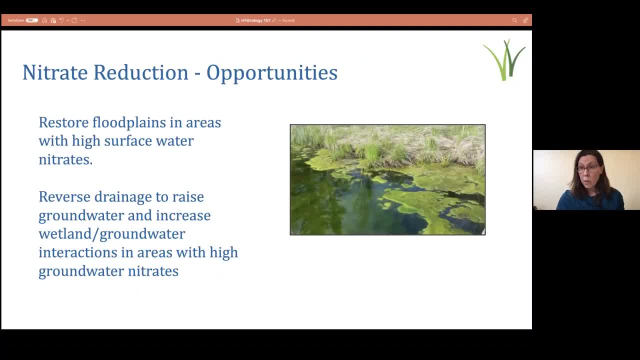 restoring wetlands to reduce nitrates. we're going to be looking for ways to um really maximize how much of our um stream systems are interacting with the floodplains in the system or, excuse me, the wetlands in the system. So, um, we might be looking to restore floodplain. 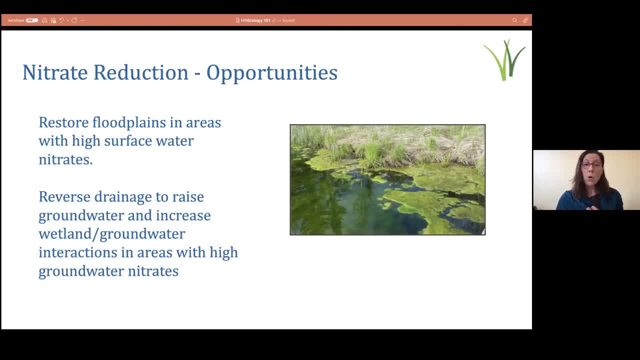 floodplains and areas with high surface water nitrates, or to reverse drainage to increase um, the way that the to to bring up the groundwater and increase the interaction of that water with the um, with the wetlands, in areas where we have high, high groundwater nitrates. 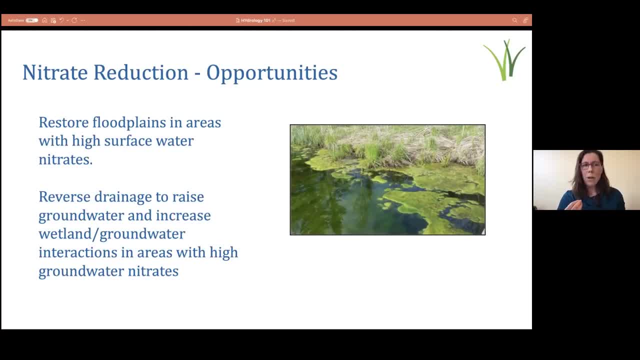 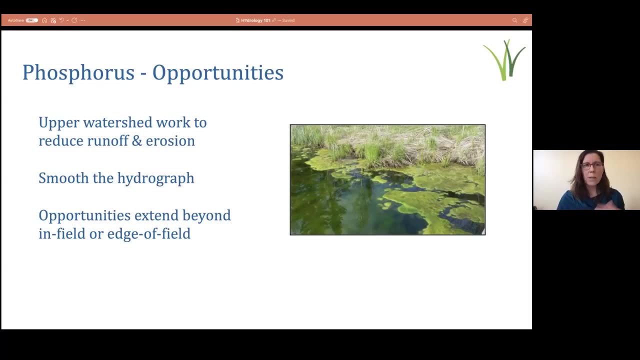 So again, uh, get that, get, get that nitrogen laden water interacting with um the wetlands and the soils and the bacteria they're in. It's a little more complicated with phosphorus And I know you all understand this because we've all been part of conversations about is it a source or is it a sink, And the 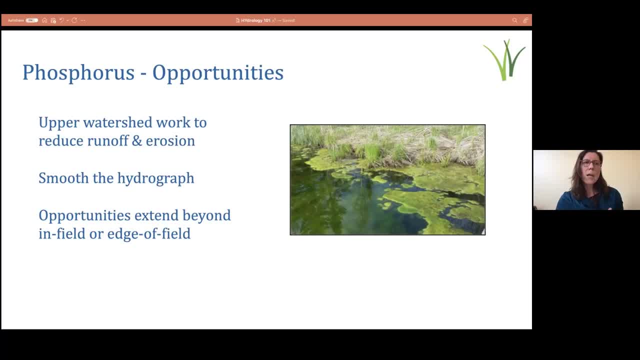 and the and. the thing I want to emphasize today is that I mean, with all of these practices, but particularly phosphorus, we really need to take a step back and thinking and think about sort of watershed scale practices. Um so, with phosphorus, 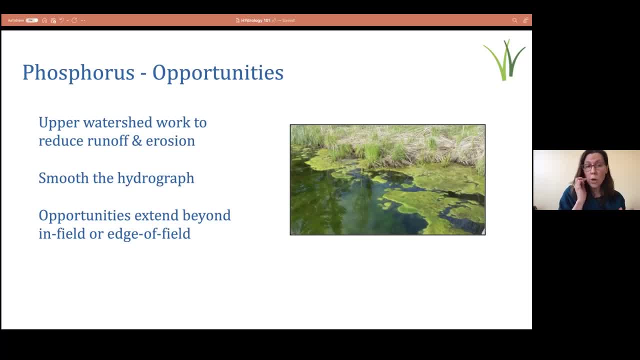 uh, you know, we want to be focusing on upper watershed work to reduce the runoff and erosion, because, of course, the phosphorus is mobilized, either it, you know, suspended in the water or attached to soil. So if, if so, if we, if we reduce that runoff, um, we can help smooth that. 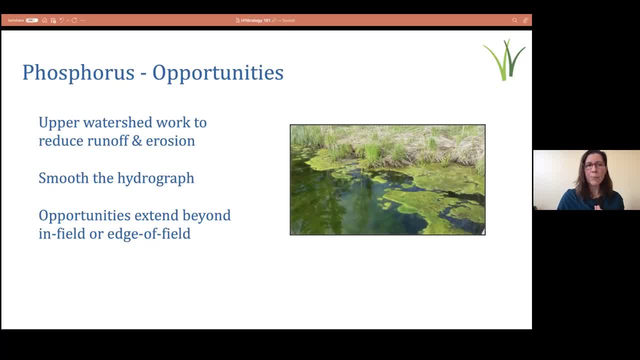 hydrograph and those things that contribute to the um loading or movement of, of of phosphorus. Um, the thing that's really nice about this is that it it means we have opportunities beyond our infield or our the edge of field practices to start to um, help manage or or reduce the the phosphorus. 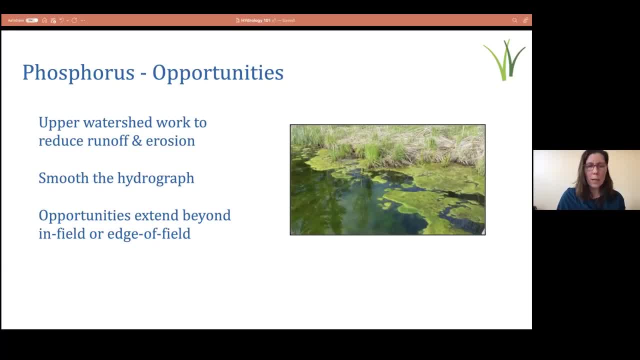 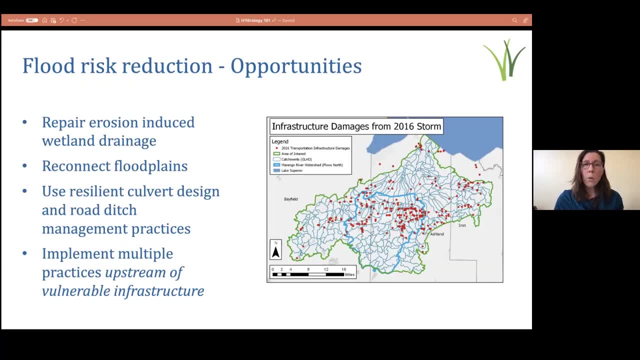 pressures in our landscapes. We need both. you know I'm going to keep saying that we need both. If we're looking at flood risk- flood risk reduction- um, we might be thinking about repairing some of that erosion induced wetland drainage, reconnecting floodplains, And I know 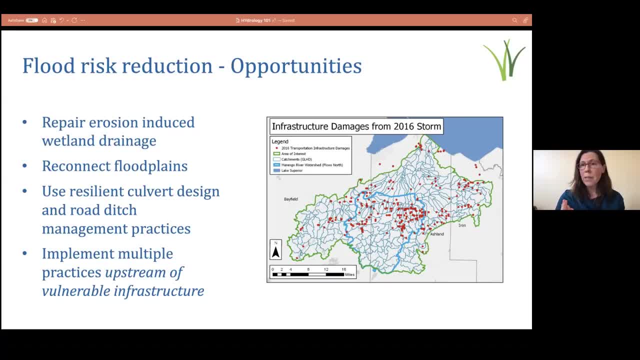 you're going to start to see redundancy here, And the reason is because a lot of these kinds of practices have multiple, multiple benefits. Um and I- I want to talk a little more about that later, but the idea here is that, um, we can spend $1 and achieve more than one thing, And that's um, that's different. 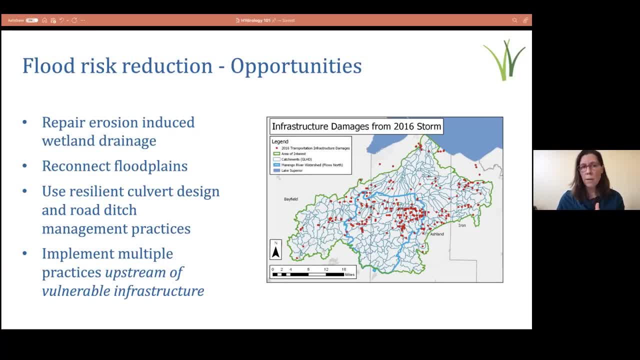 than some of our interventions which are really designed to do one thing at one site. Another thing with flood risk reduction is um we have opportunities to improve our culvert design or a road ditch management practices to have a a a better influence on some of the hydrology and 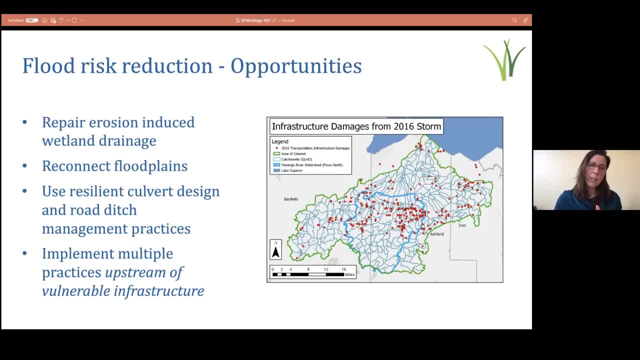 geomorphology, And so, um, we have opportunities to improve our culvert design or our road ditch management practices to have a better influence on some of the hydrology and geomorphology that's needed to have healthy stream systems, and location, again, here really matters, So you might think about. 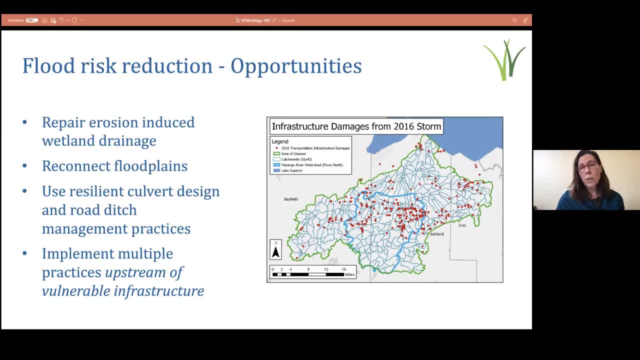 implementing multiple practices upstream of vulnerable infrastructure And um, and that's really the target of the um, of the work that's going to be described in the technical roundtable that follows this session. And then groundwater recharge opportunities. here we want to really 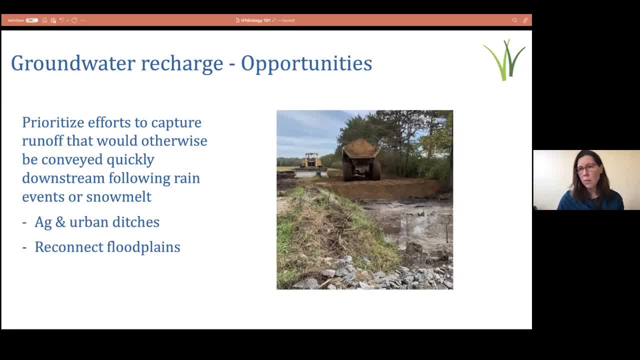 prioritize efforts that capture that runoff that would otherwise be conveyed quickly downstream following rain events or snow melt. So, um, we have opportunities to improve our culvert design of as far as housing infrastructure- and that's a little bit of both, considering tailoring and. 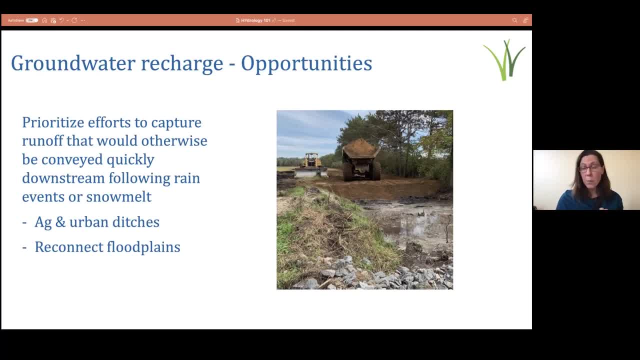 aggregating 'll also mehrlaughs gesZ. we're really, really important and really helpful to be thinking about where there's opportunity to um restore them and, and you know, something that's important to know is that, um we have a lot of legacy ditches от. 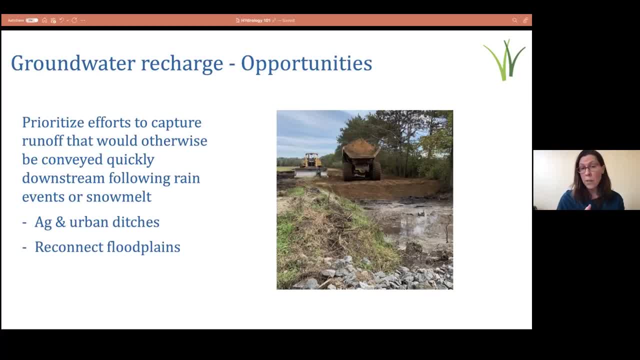 things that were put on the landscape 100 years ago and aren't really serving any functional purpose today. Obviously, a lot of our ditches are still supporting active agriculture. Only operational operations. Fancy Creek that I showed, that channelized stream with the meandering channel, that ditch is not. 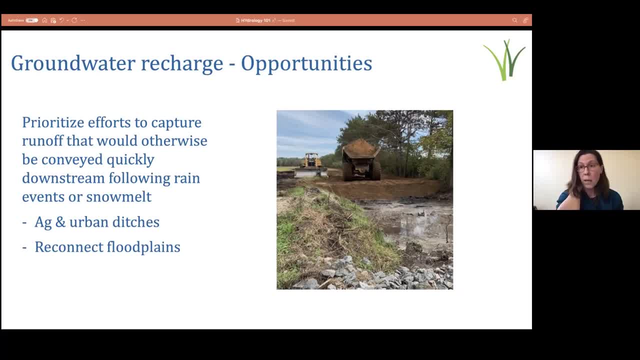 serving any purpose and the landowner doesn't really want it there anymore. So it's a great stream restoration, floodplain reconnection opportunity And then, of course, groundwater recharge, also reconnecting floodplains so that water can come out of the stream, move out across. 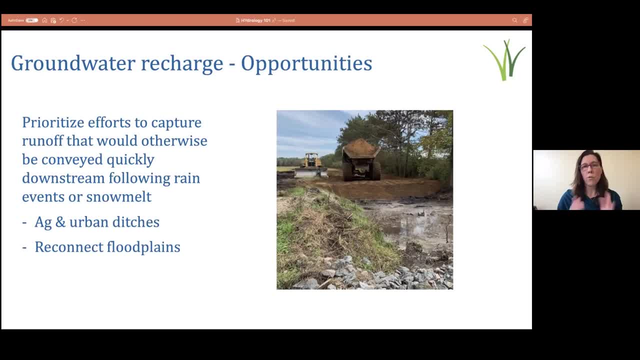 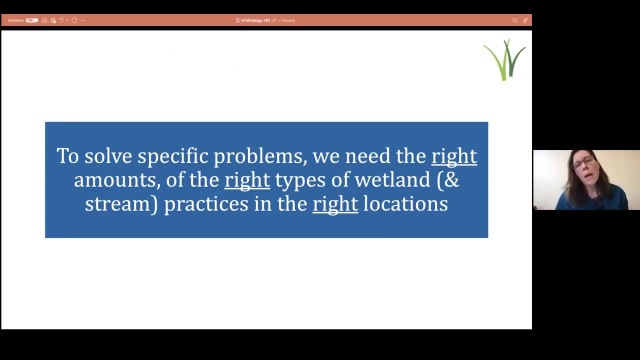 the floodplain, sink back in and return to the river right there in a big loop, as opposed to going straight downstream and being lost forever. Okay, So another one of our mantras: to solve specific problems, we need the right amounts of the right types of wetlands and stream practices. 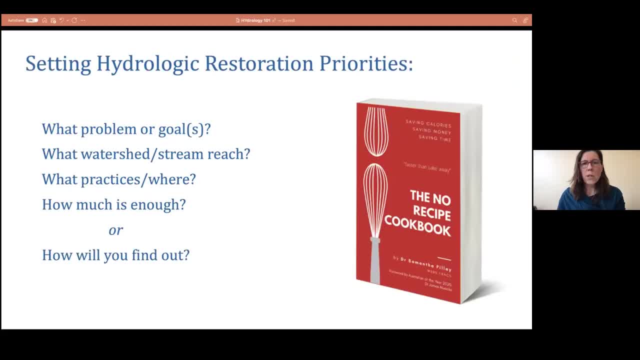 in the right locations. So I want to pivot here and talk about what this looks like in the context of a land and water management plan or any land management effort. So when we're setting hydrologic restoration priorities, there's really no cookbook right, It's not? 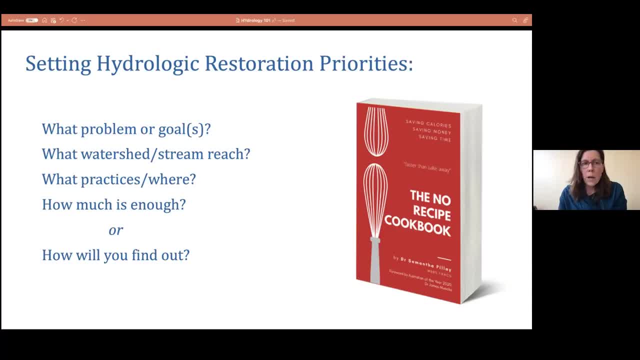 you know, it's not put wetlands willy-nilly anywhere and benefits come what may. We want to be thinking about what problems or goals we're trying to address, what watersheds or stream reaches we're looking to restore, what practices, so what kinds of wetlands or what kinds of stream practices, and 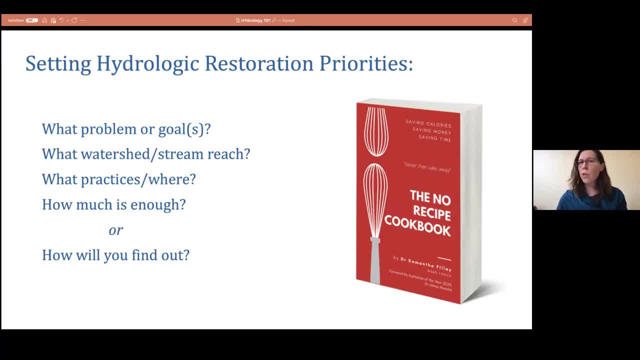 where, specifically, how much is enough or if you don't know what's your process going to be to find out. So we've had the opportunity through some of our work- particularly, excuse me, an EPA grant- to look at a bunch of county land and water management plans and the wetland content in 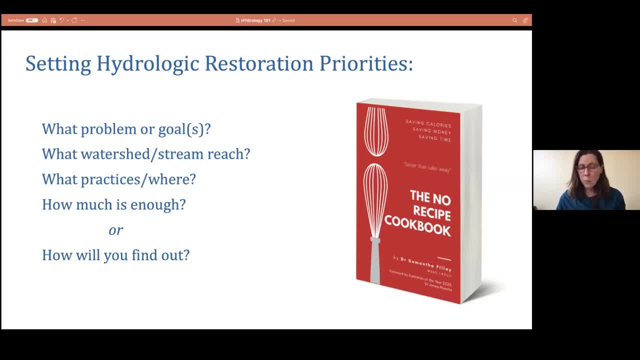 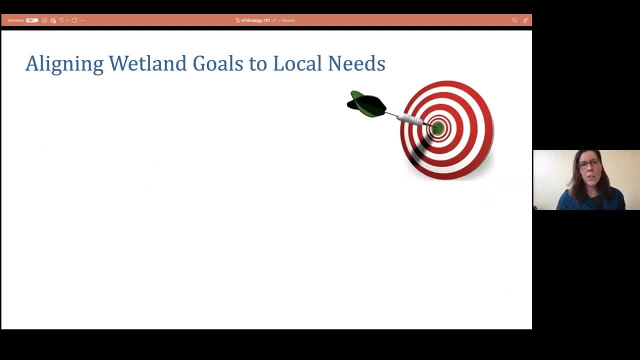 those plans is really variable, So I've taken the opportunity to paraphrase a few things that we've seen in some of these plans. I'm not going to call out or name specific counties, but I want to talk about opportunities to better align our wetland goals. 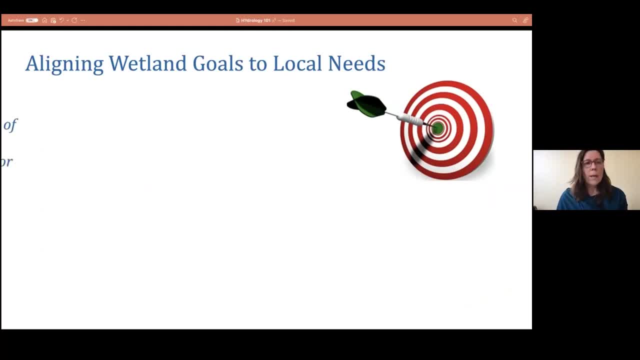 to our needs or the problems we're trying to solve. So here's one example: Promote development of new wetlands and restoration of drained or degraded wetlands. Well, it doesn't say where, and it doesn't say for what or how much, So this is a fairly generic goal. Another one we found was: 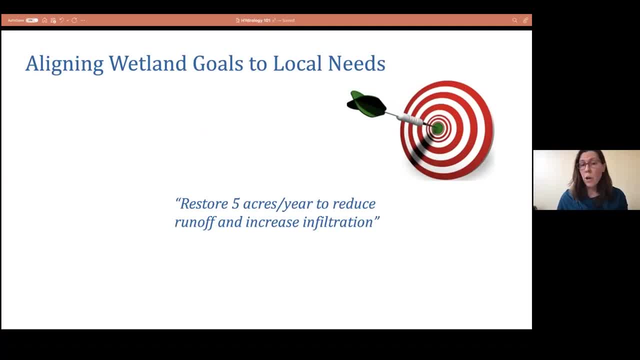 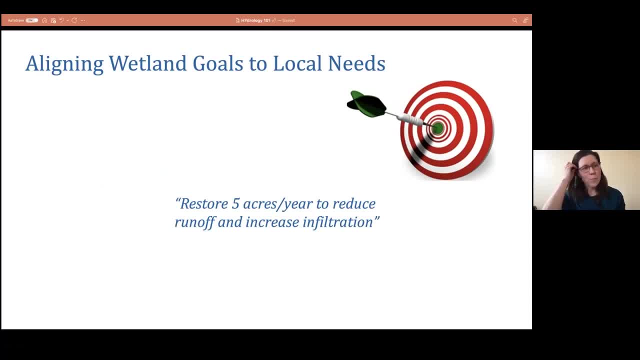 to talk about what we're trying to do. So we're going to talk about what we're trying to do. So this is a measurable target in terms of acreage. That can be a lot in a situation where you might just be looking at prioritizing a specific flood plain. It's not very much in the context of an 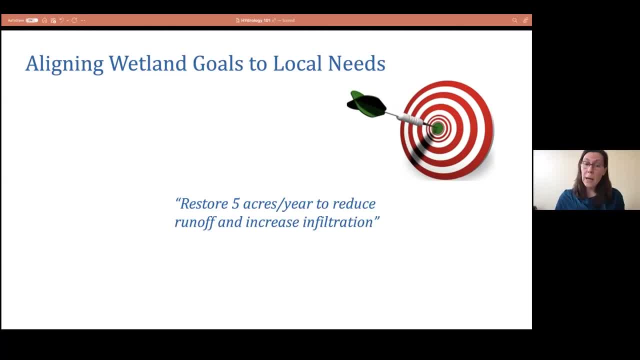 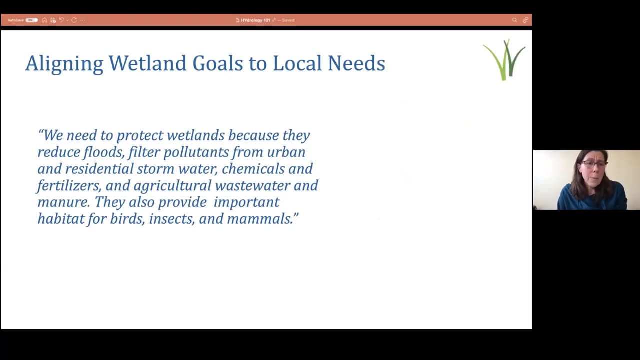 entire watershed. but it's good here that we have a goal: reduce runoff and increase infiltration. We can improve goals like this by just being more specific about what or where or how much. Here's another example, And I and I- And this is a paraphrase from an actual plan, I cut it down a little bit, but we need to protect wetlands because they reduce floods, filter pollutants from urban and residential stormwater, chemicals and fertilizers and agricultural wastewater and manure. 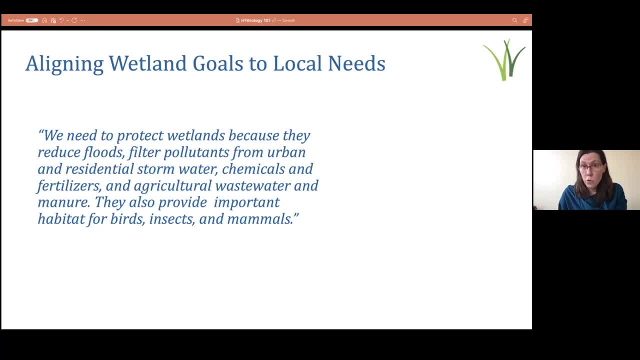 And they also provide a lot of habitat. Well, these are all true. It's one of the reasons we love wetlands, But this statement is really more of an educational statement or reflective of a value. We need to protect wetlands because they're important, but it doesn't really get at. you know again, for what or for where. 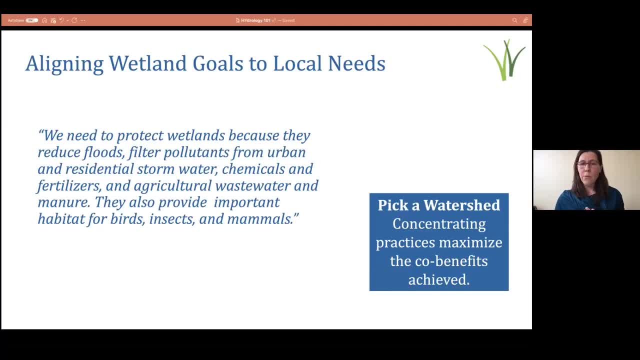 So a recommendation I would have is, if we're really looking to maximize the co-benefits that wetlands achieve, we can pick a watershed and we can concentrate a variety of wetland practices across that watershed so that we can get at all of the 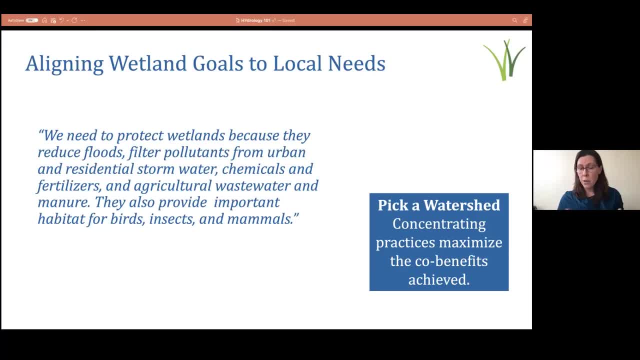 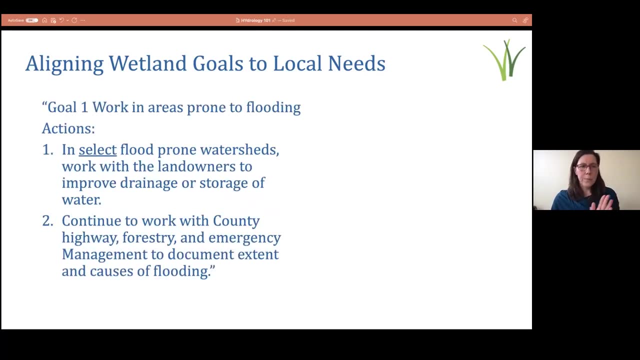 these beneficial functions that wetlands provide. It's another approach if you want to be more inclusive of what kinds of wetland functions we're looking to restore, what kinds of problems you're trying to solve. So my last example moves things along a little bit. So work in areas prone to flooding And the actions are in select watersheds. work with landowners to improve drainage or storage. So we've got wetlands. 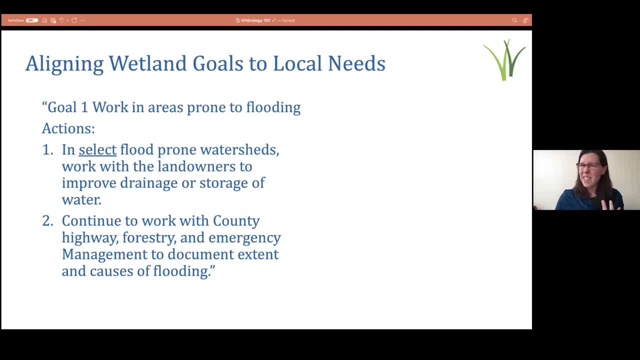 What's our goal? Flooding Where, Select watersheds. It doesn't name them, but that's okay because it's saying you know where we have flood prone situations, working with who to do what, drainage and storage. 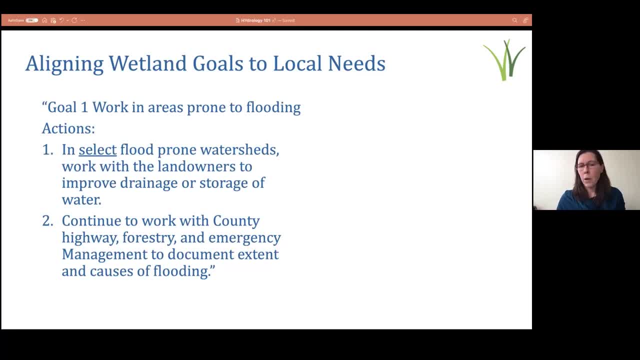 And- and I really like this part- continue to work with county highway forestry and emergency management to document the extent and the causes of flooding. So I think this is really well done. It recognizes that there is a problem, that we don't know everything we need to know about a problem, but sets 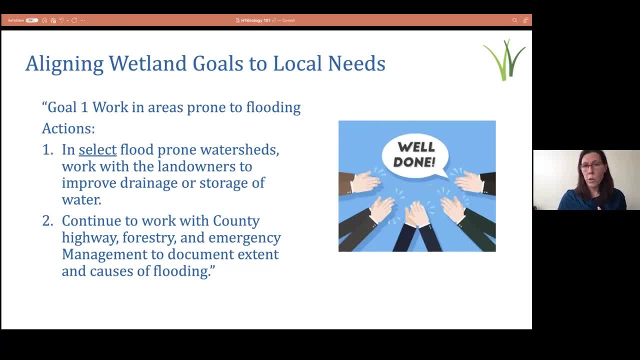 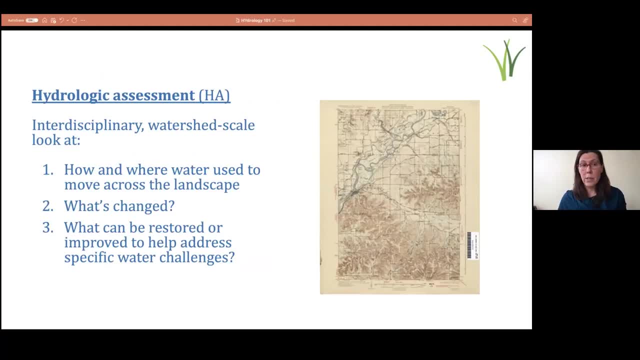 So I think this is really well done. It recognizes that there is a problem that we don't know everything we need to know about a problem, but sets And- and I really like this part- continue to work with county highway forestry and emergency management to document the extent and the causes of flooding. So I think this is really well done. It recognizes that there is a problem, that we don't know everything we need to know about a problem, but sets 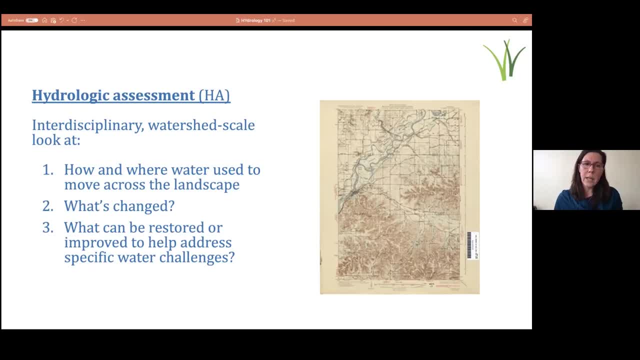 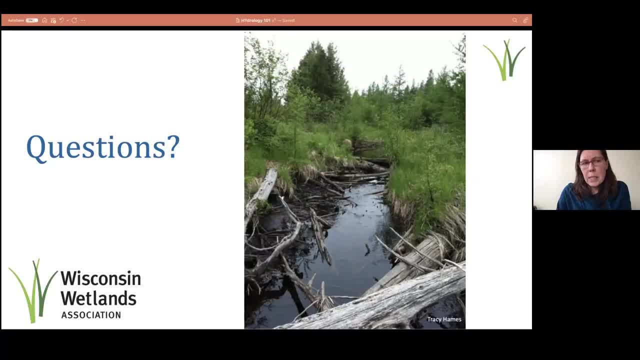 Hang on. I'm going to have to punt on that question because it's not my area of expertise, but I will Hang on. I'm going to have to punt on that question because it's not my area of expertise, but I will. I'm going to have to punt on that question because it's not my area of expertise, but I will. 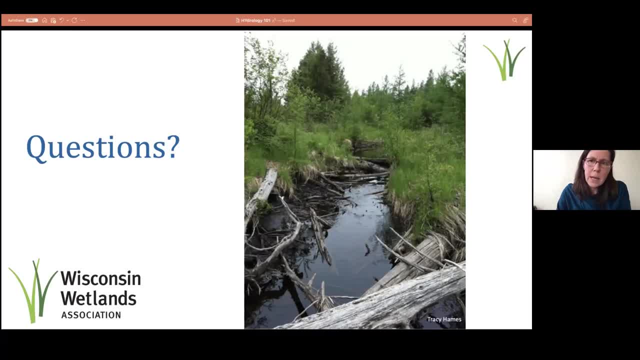 I will look at the chat When I'm done and I will have someone on our staff or appear on a Nossaomas intern or anyway. genealogy ins тест try to address that question, But I think there might not be like one right answer, because we've 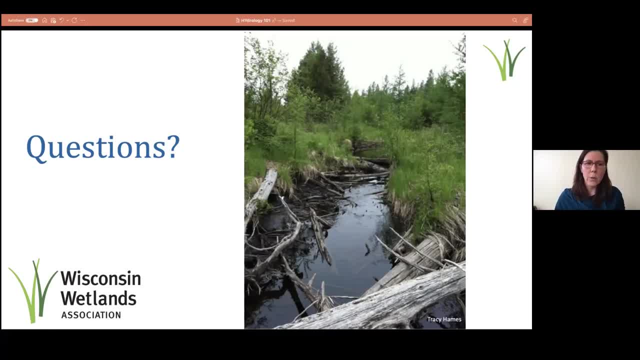 seen situations where grazing in the floodplain is appropriate. We've seen situations where grazing in the upper watershed is appropriate. So it really might just depend on you know things like number of cows and condition of the wetland. You know, maybe you wouldn't put cows in a really 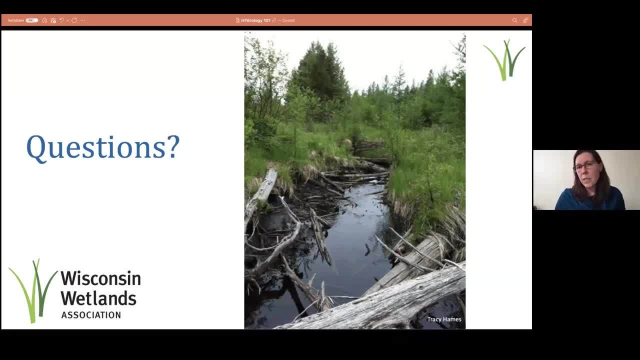 high quality wetland. but if you've got a degraded site where you need some vegetation management, that's one example where it would be really helpful. But again, I'm not sure Go ahead. Wetlands can bleed phosphorus over time as plants decompose. Can management harvest? 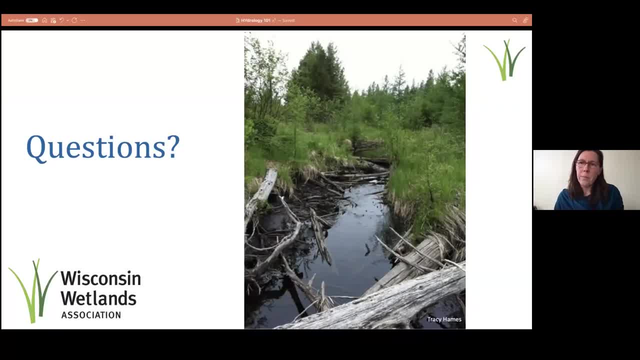 a vegetation be a viable option for removal and reduce this loss. I think that's certainly a practice that some folks are using and I believe there is some research supporting that. Again, no one right answer, So you also need to be thinking about what's going on above it. 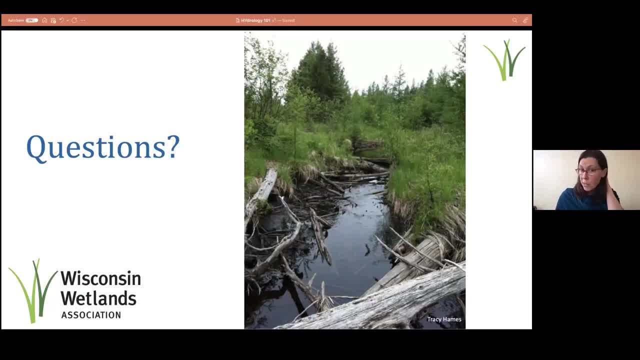 what's going on below it, But for sure, harvesting vegetation is one way to remove phosphorus from a system. In high groundwater situations, would a wetland keep up breaking down the nitrogen faster than it would be reaching groundwater? Great question, You know we do. 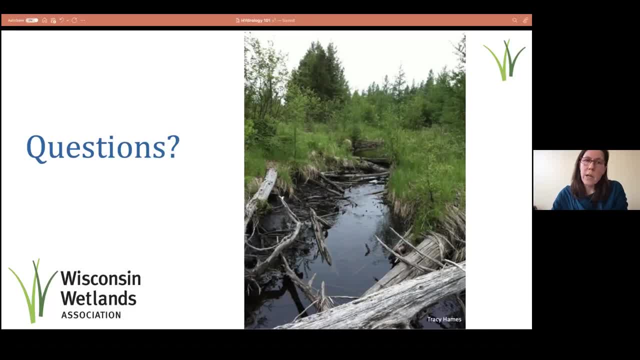 we do need more research on the finer details of nitrogen management or denitrification, particularly when it comes to situations where there are higher groundwater nitrate concentrations in groundwater. So you know I can't answer that question without looking at specific studies, but I can say that the properties of the wetlands do support 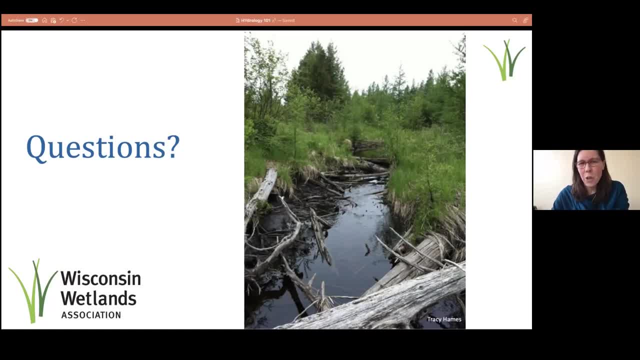 denitrification, How much, how much wetland we need, how much groundwater we, how much amount of water it needs. So we need to address these questions And I think that sort of interaction we need to achieve those objectives, I think is something. 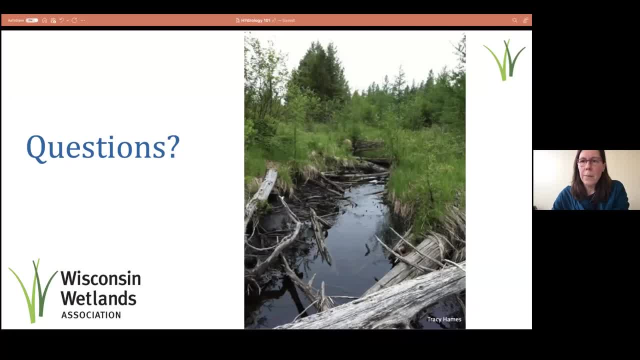 we need to study and we need to test. You want to continue? Yeah, we can take a couple more. Okay, Are you seeing counties and or the state consider mean to prevent deforestation and land disturbance in wetlands and the areas surrounding them by utilizing county zoning wetland districts? 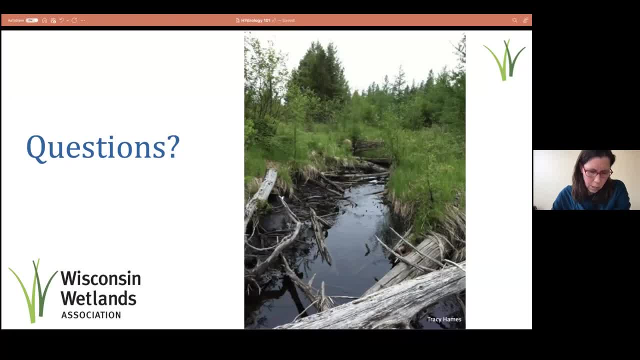 Well, it's a high number on the district. That's not what I think it's going to be, but it's okay, I think it's not. Well, there's, there are definitely land use zoning tools that can be used to prevent conversion of forested wetlands to other uses. 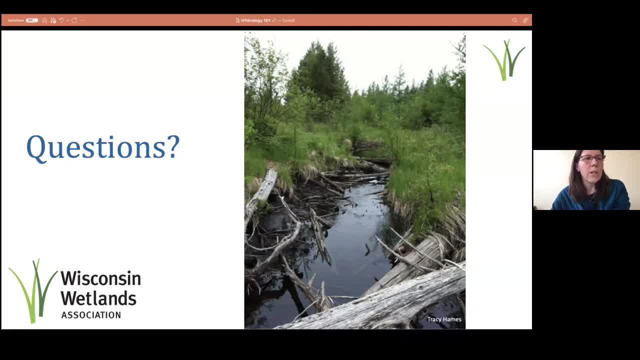 You know, protection, preservation is an incredibly important tool in the toolbox. It has limits just because of what we can achieve. you know, socially some counties are going to be more inclined to use land use controls than others, But I think we should be. we should definitely be. it should definitely be in the mix. 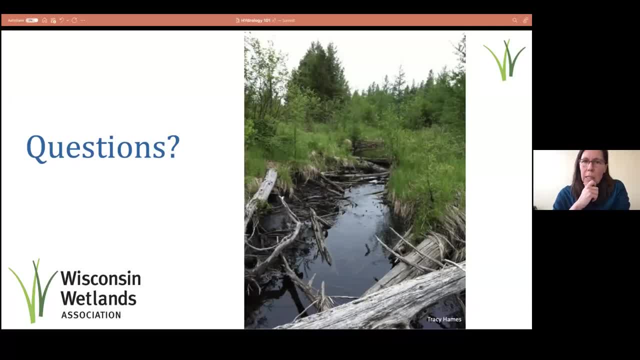 It's been a while since I've looked through specific zoning policies to give you, To give you, examples. So we did do some. We did do some summaries of zoning controls on wetland development and stormwater policies 10 years ago or so, but I don't have specific examples here for you today. 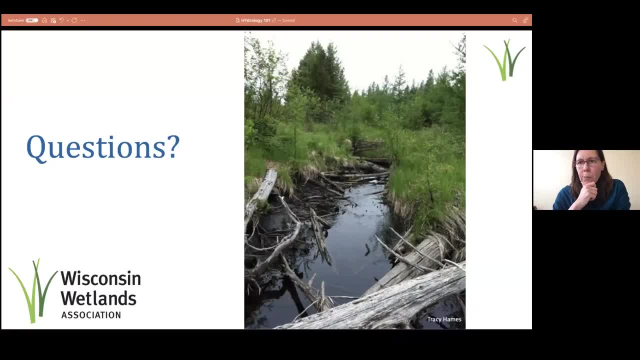 Can you touch on prescribed burns and their benefit or harm to how wetlands flow? So I think this is a good time for me to say: you know, I'm the policy person, right, I have a science background but I'm not a practitioner, And so there are probably others on the on the call that have more direct experience. 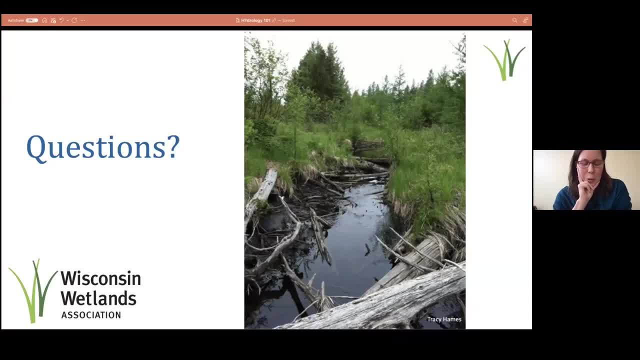 I've got some fire management experience from 20 years ago. but you know, fire is a another management technique, just like grazing, just like mowing, And in the right situations it can be very helpful. You know it's also. 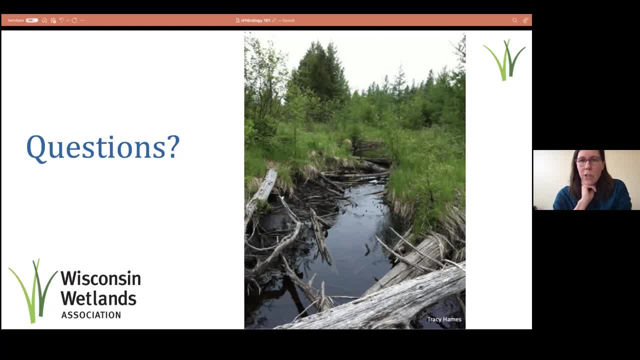 true that that standing vegetation provides friction and can help slow flow, so, um. so, of course, there are going to be some differences on how flow. you know how flow moves with or without that standing vegetation. is it a? is it a bad thing um to burn? um, you know, maybe there is a. 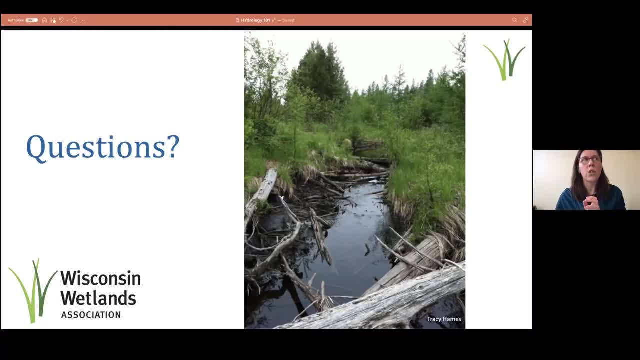 question, uh, but i wouldn't, i wouldn't unilaterally dismiss any of these practices. and what, um? if any of you have seen tracy from our office present, you know he likes to say there's no bad techniques, there's only um techniques used in the wrong um situations. and so, uh, again, it's a tool and i've 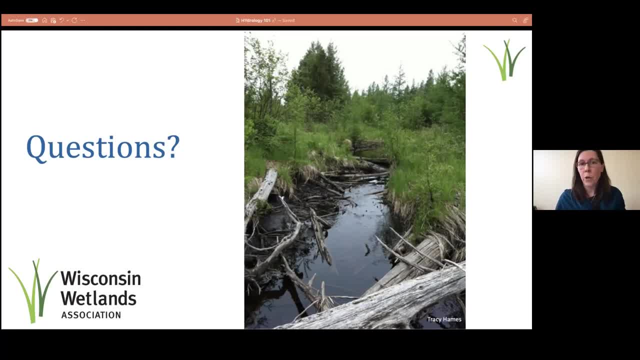 worked in other wetland systems in other states where we we did a lot of active burning and it was part of the um, part of the protocol for having healthy, healthy vegetation, and there were not concerns about effects on hydrology. let's do one more and then move on. 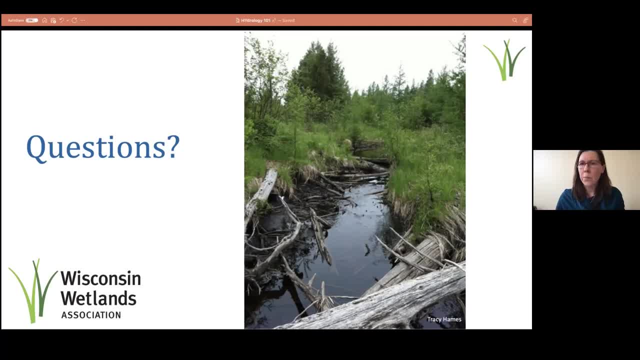 and we'll hopefully have time um at the end here for questions as well. uh, i just want to point out before i read the last question, kate brenner put in there the flow. the flow is the next conference session from 10- 15 to 11: 30. so yeah, thanks, um, you have. 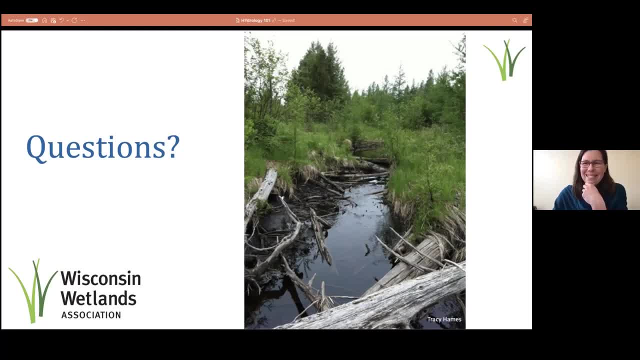 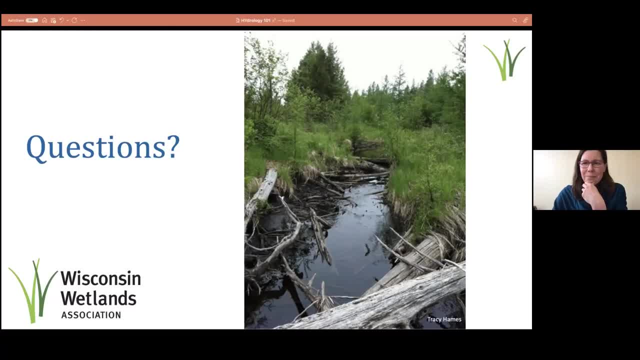 rural landowners are faced with in regards to wetlands is how they are being assessed by tax assessors. being taxed as recreational land, therefore, the farmers drain or pasture them, so they so the wetland is assessed as ag land. what can a farmer do to make sure a wetland is? 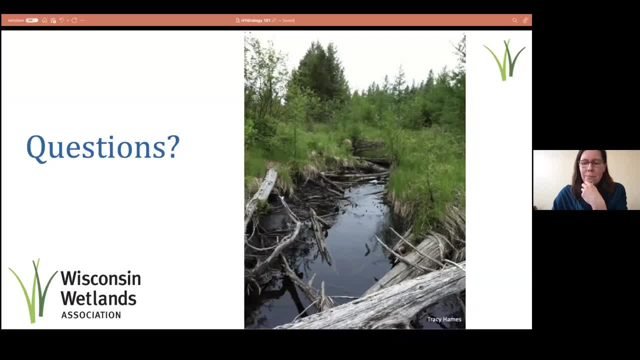 not assessed as recreational land but as an ag land or some other land use? yeah, so a great question and actually an issue i've worked on a lot over the years. um, any wetland that has a compatible agricultural practice on it- haying or grazing is an example. 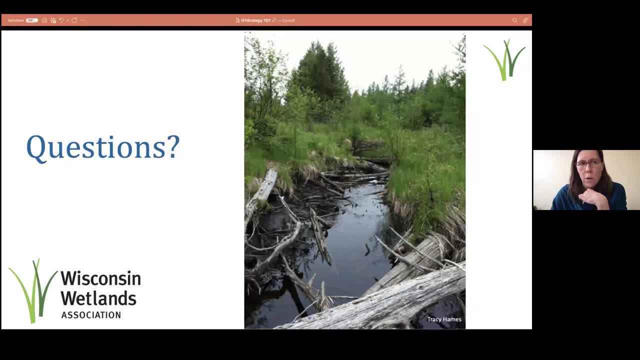 um as a management practice is going to qualify for um agricultural use taxation. if it's strictly recreational land, it's going to be taxed at 50 of fair market value. um. so there's still a break there, but not uh. it's not quite as low as as agricultural use value taxation. so having uh. 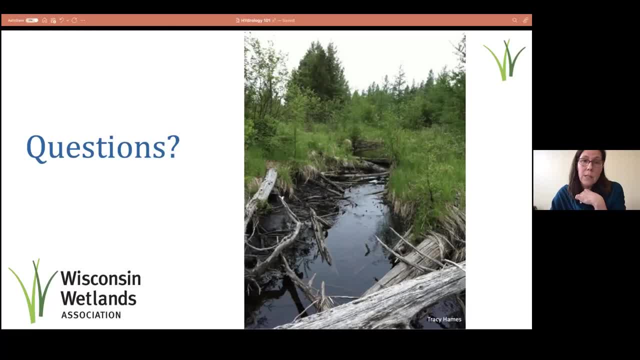 having a wetland, having a managed wetland in a farmland is going to be taxed at 50 percent of fair farm landscape, with some um remaining. compatible agricultural uses is one is one opportunity, um, and i think i'll leave it there, but if you have more questions about that, please, 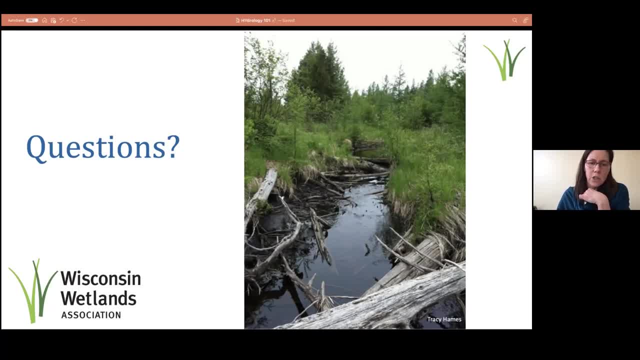 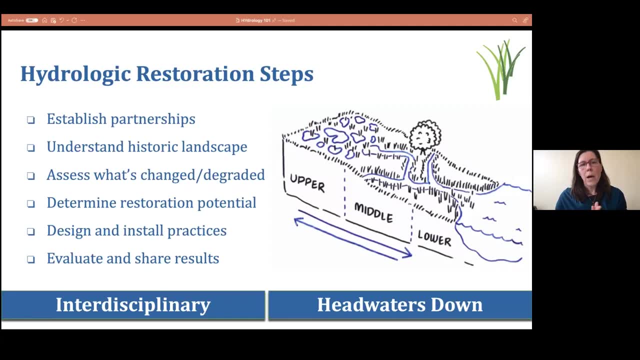 contact me and we can talk. we can talk in more detail after the session. okay, so i'm going to move into some quick case studies. you know, when we think about putting all this together, um, there are are steps that are somewhat formulaic, although the work itself is not. 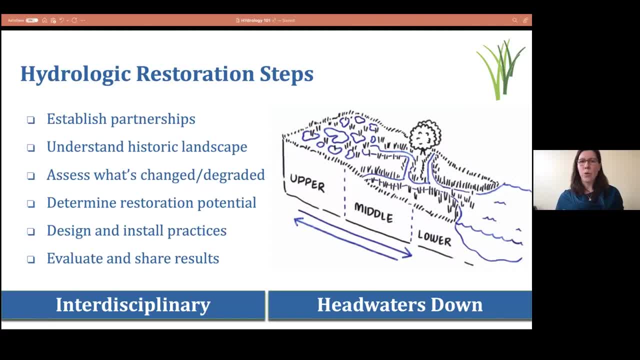 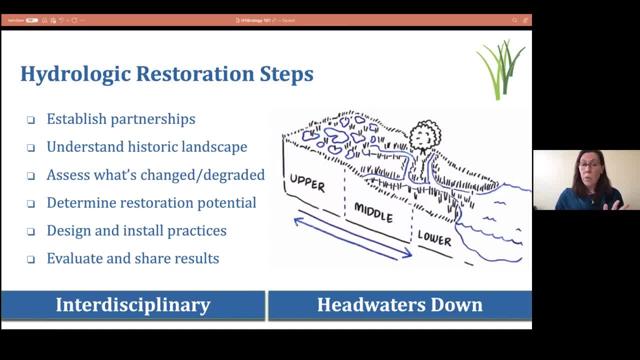 landscape and assess what's changed or what's been degraded and to what effect. we need to evaluate and determine the restoration potential of, you know, specific sites, um or specific catchments, design and install appropriate practices to address those process um issues or to improve those processes. and then, of course, we're going to move into some of the next steps. 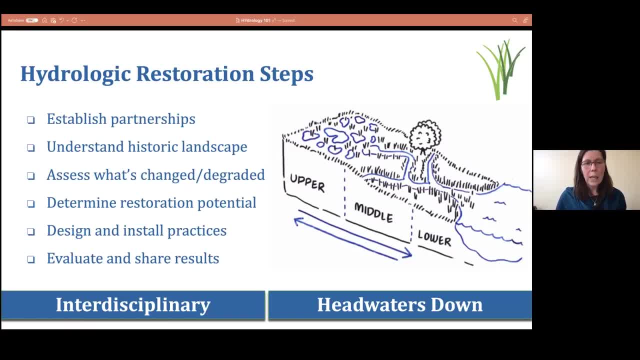 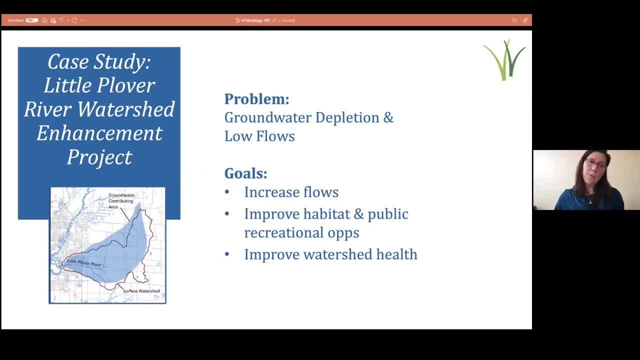 to evaluate and share results so that we're all learning, and i want to use this case study from the little clover river watershed as my example. i'm not going to get into the specific practices that have been implemented or the results of those, except to say that we've been doing a lot. 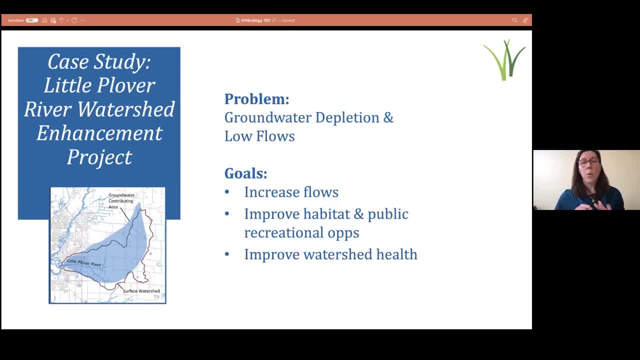 of restoration and the results are very positive. but i want to talk about the structure of the partnership and the problems we're trying to solve and how we've approached them. so the problem in this watershed- if you're not already familiar, most of you are- is groundwater depletion and 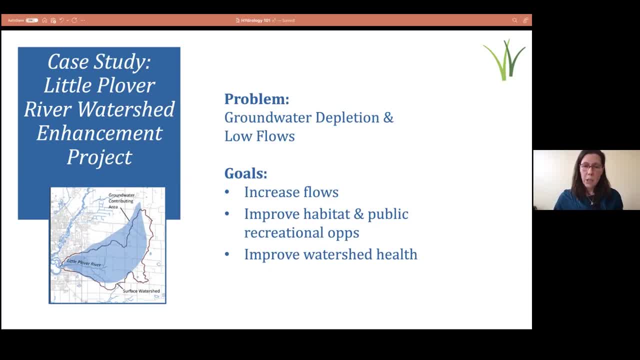 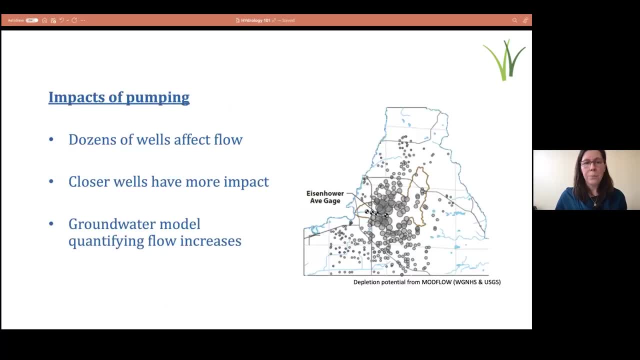 low flows, and the goals of the enhanced water system are to ensure that the water is not depleted, the water is not out of theatanic and the water is not void. the actions of the different areas are to increase flows, improve habitat and public recreational opportunities, and improve watershed health. 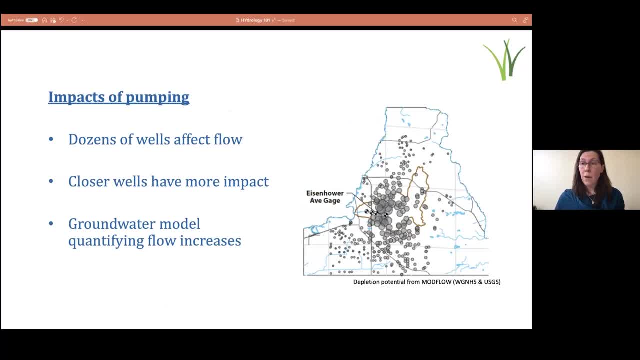 this watershed is infamous because, um, we've had a lot of high, uh, high capacity wells go in near the river and it's uh and it's uh, it's lowered the groundwater table and had a very significant impact on flows. we have good models, um, that tell us that it's dozens. of wells that are affecting the flow in this watershed, and that's because we have high capacity wells that are affecting the flow in this watershed, and so that's why we're working to address that. and i would really highlight what the яweri project is all about. 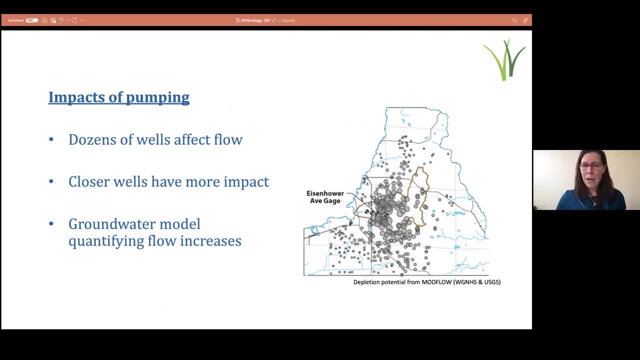 this river. The wells that are closer to the river have a higher impact, represented by the larger circles on this graphic here, And we have the model that tells us how much flow we'll get returned to the system by removing any given well or any given cluster of wells. It's a great. 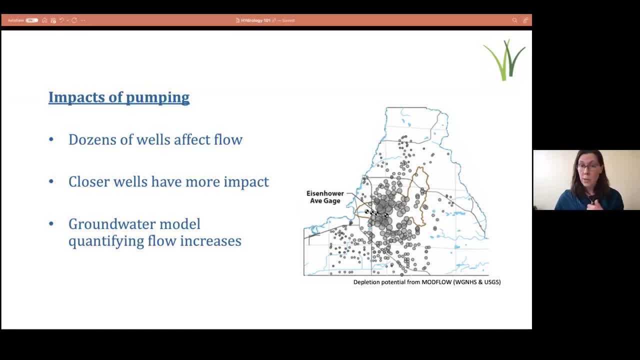 example of where we have good data that looks at a specific contributing problem and allows us to make recommendations on what needs to happen to address the problem. So in this case, I think they recommended, you know, if we moved 10 or 12 of the wells closest to the river, took them. 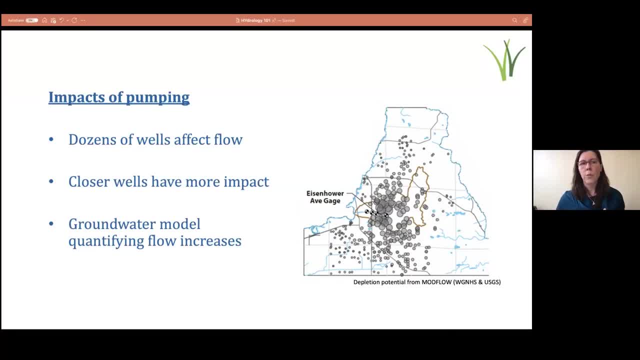 offline, we could, you know, solve the problem or the majority of the problem. all things equal and not changing. You look at something like the Central Wisconsin Lake Study and I think the recommendation was, you know, remove 300 wells and we'll get the groundwater back in those lakes. 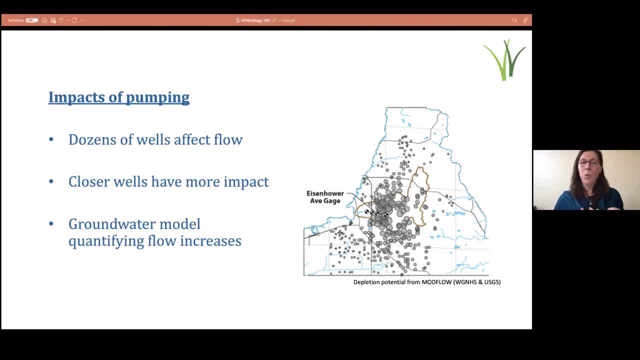 That is an example of where the science tells us what we need, but it's not necessarily a realistic goal, because we don't have 300 wells. We have 300 willing landowners or 300 operations that are willing to take their wells out. 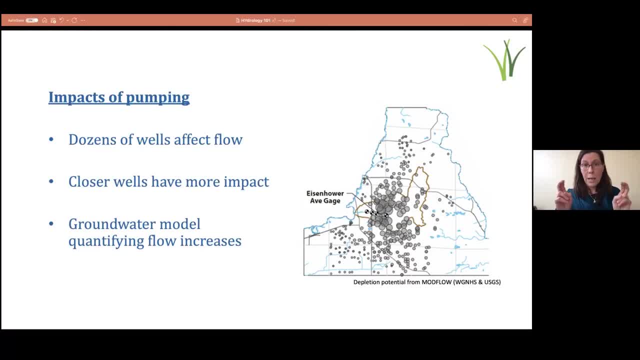 Another example of where the data might give us. you know, the answer would be: if we convert 80% of our cropland to grassland, we could solve, you know, whatever runoff management problem. Well, again, the numbers add up, but it may not be a viable solution. So we need to look at. 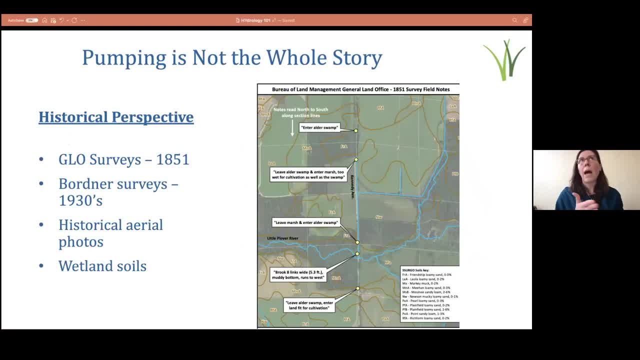 what else is contributing to our problems or what other avenues or pathways we have to address them. So in the Plover watershed, pumping is not the whole story. When we go back and look at the historical landscape, we have really good information and you all have this for every watershed you're working in from. 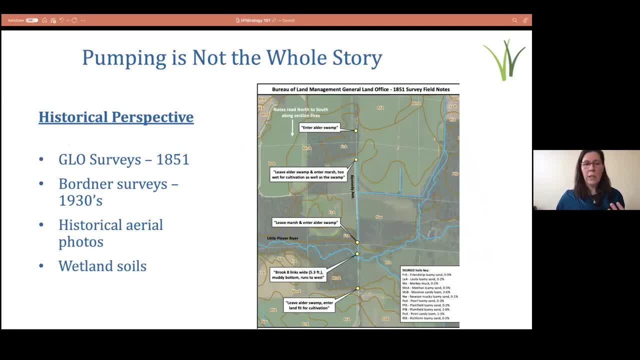 surveys dating back to the 1800s and the early 1900s. historical photos, our wetland soil maps that give us a better feel for what that landscape looked like before it was developed for agriculture or other uses. Very detailed and specific information about the hydrologic system. 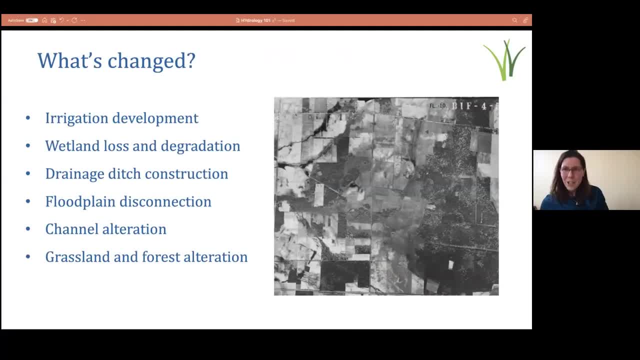 And when we look at the question of what's changed. in addition to irrigation development, there's been a lot of other changes. We've lost wetlands through ditching and drainage. The floodplain of the river is disconnected. The channel has been widened and made more shallow. 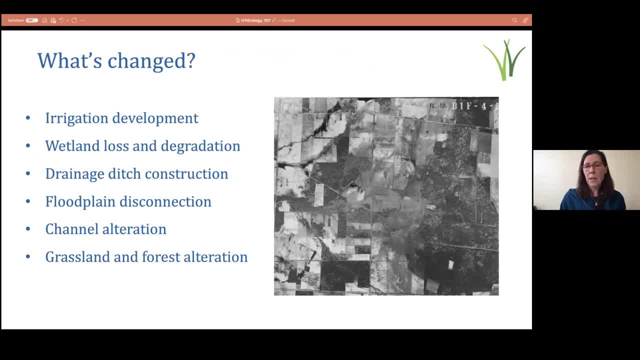 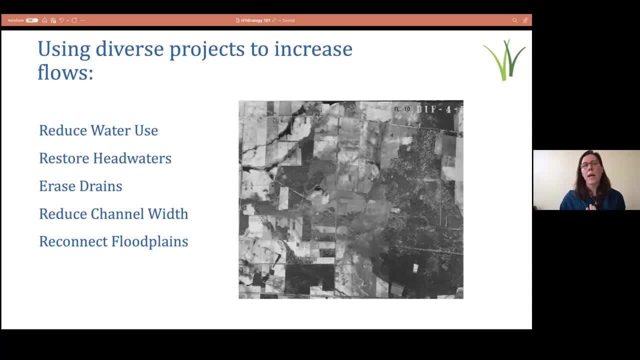 And there have been a lot of other upland practices that have affected hydrology drainage infiltration. So what this does, when we look at this more holistically, it allows us to use diverse projects to increase flows. So reducing water use is a very important part of this. 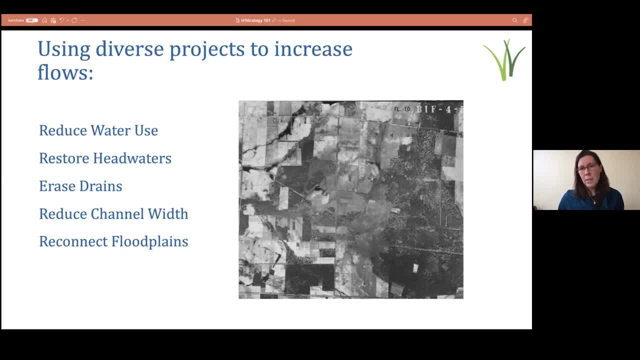 It's a very important part of the practices that we're employing in the Little Clover River Watershed, both decommissioning of some agricultural wells but also adjusting pumping regimes of municipal wells. And then the village of Clover is also looking at repairing leaks in its wastewater return systems. 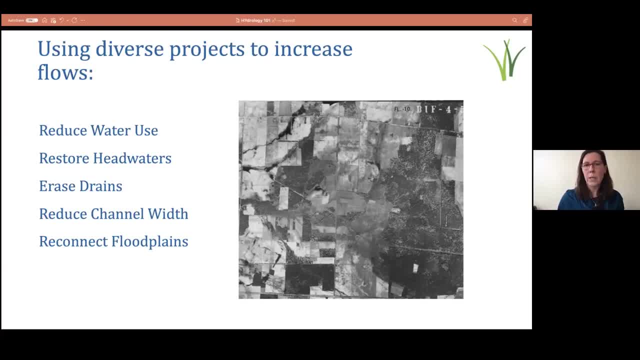 because there was a lot of water that was just leaking out of pipes that were in disrepair and going downstream. So we're recapturing and holding on to that water, restoring headwaters, erasing drains, reducing the channel width, reconnecting the floodplains. 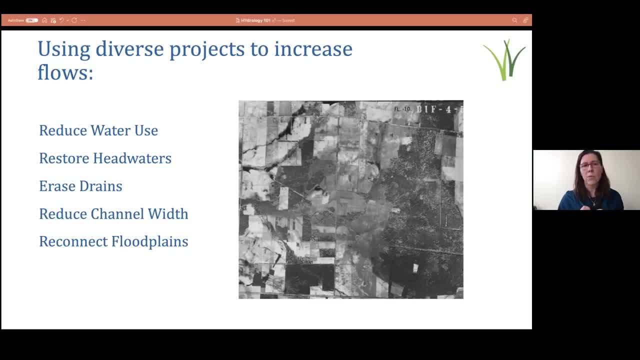 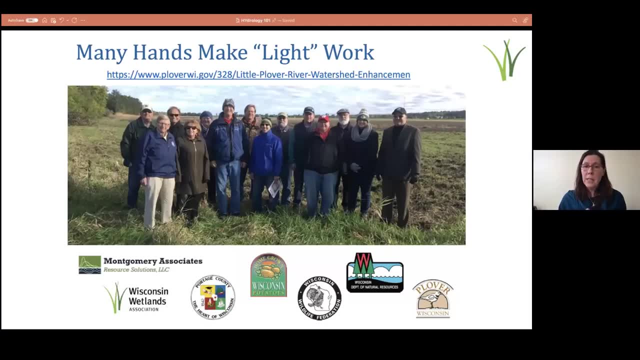 And each of these practices incrementally is having a positive, beneficial impact on the flow And we're getting a lot of other co-benefits in the process. So the message here in this case is: many hands make light work, Many practices make work feasible. 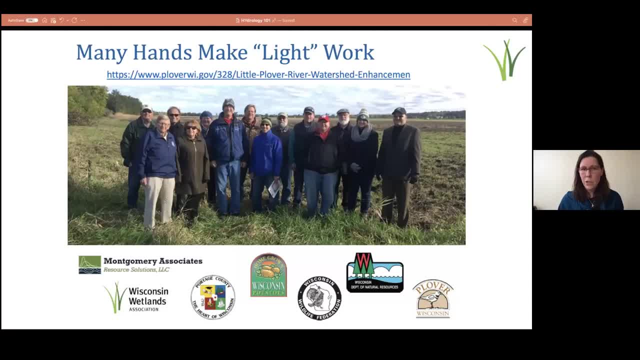 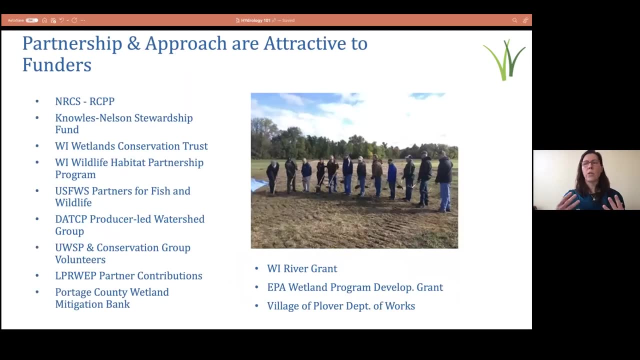 In this case it's an interdisciplinary, intergovernmental, public private partnership between the village, the farmers, some statewide and local conservation organizations, the county and others, And when we have this robust partnership- and yeah, we are 950.. Okay, thanks, I'm almost done. 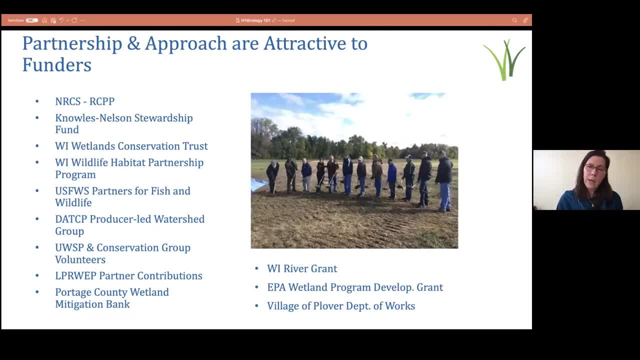 When we have the good, the good plans and the good collaborations and a lot of partners at the table, the funding, the funding is the easy part. Finding funding for restoration work in this context is is it takes. it takes capacity, because we have to write grants and 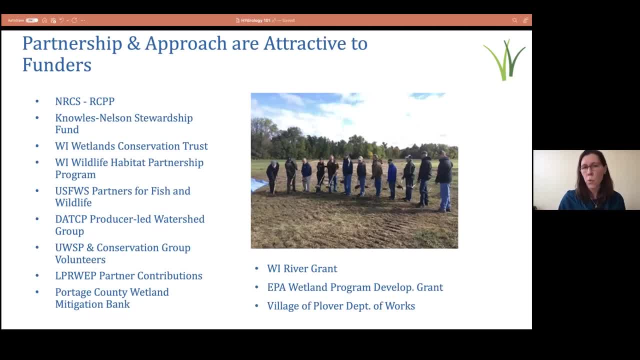 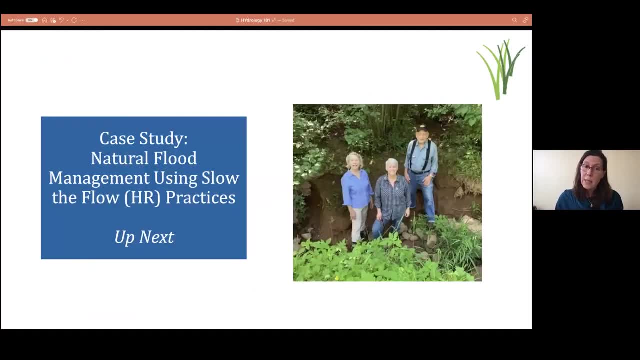 manage those grants, but the finding the funding itself for the work itself is is really very simple. I'm not going to give a lot of details about this, but I just want to mention- and I think Megan's going to put another link in the chat- that that the the other case study, that 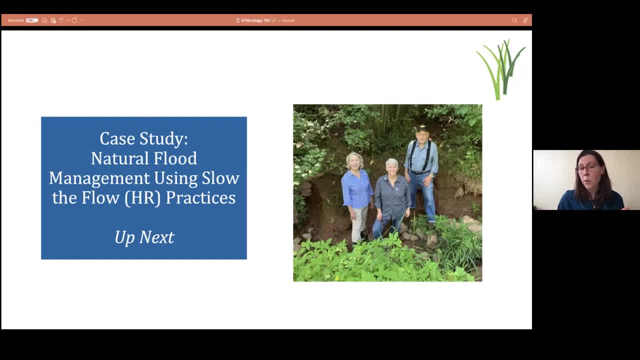 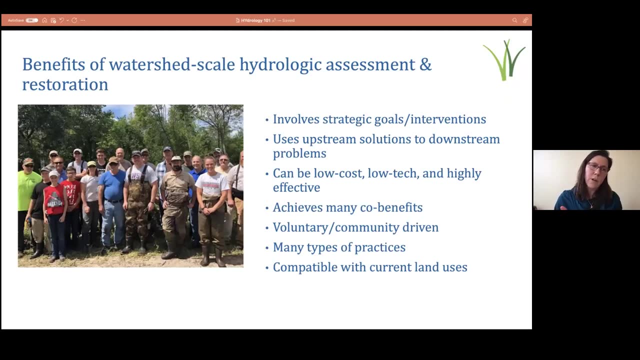 we're working on pilot project is the natural flood management using slow-flow practices in the moraine River watershed in Ashland County, and that's, of course, the topic of the next of the next session. So to to wrap it up, and if we have time in the final minutes of our discussion, I'll talk. 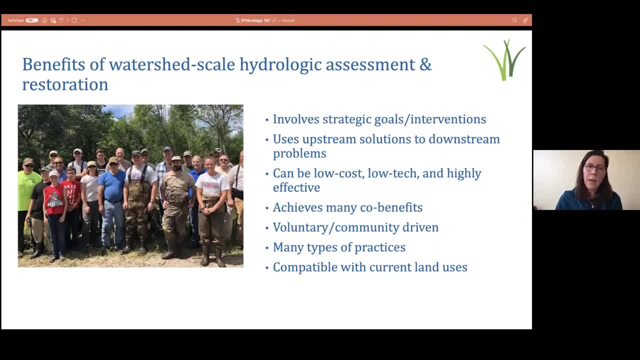 a little bit about some of the things we're doing next. but benefits of this watershed scale approach to hydrologic assessment and restoration is that it involves strategic goals and strategic interventions. We're using upstream solutions to solve downstream problems which can be very can be low cost, low tech, highly effective. It achieves many co-benefits. The work 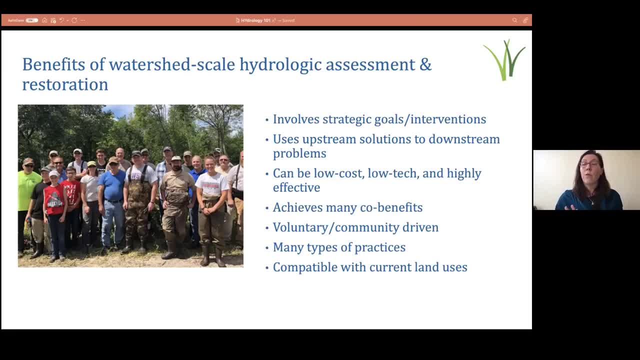 can be voluntary and community driven. We have a much broader toolbox in terms of the kinds of practices we can use to try to address these problems, And the work can be done in ways that's compatible with current land uses. So some of this work can happen on working farms or on lands. 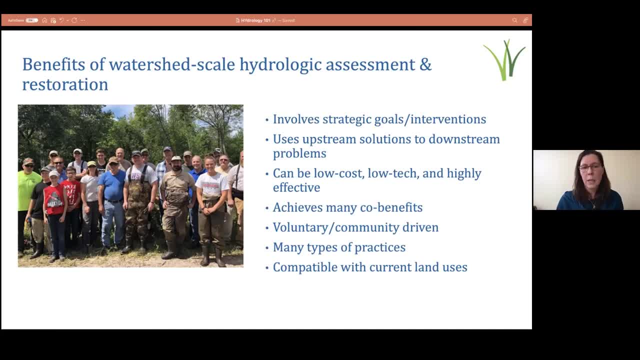 that aren't agricultural lands. Some of this work can happen in urban landscapes. So it's really a matter of understanding where the problems are, where the opportunities are, and there's just a lot more opportunity to engage landowners in in the process and along the way. So with that, we 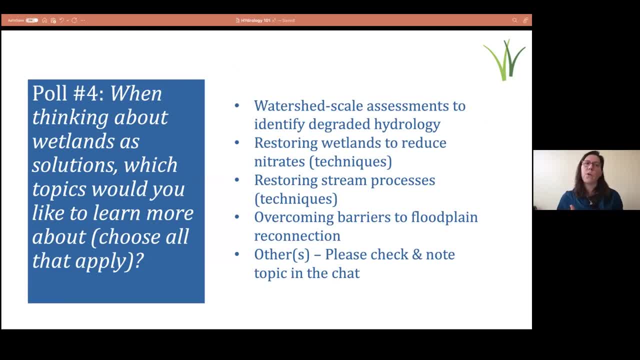 have a final poll, kind of trying to get a feel for have we whet your appetite here And what would you like to know more about? I think the questions in the chat also give us an indication, but when? when you're thinking about wetlands as solutions, which topics would you like to learn? 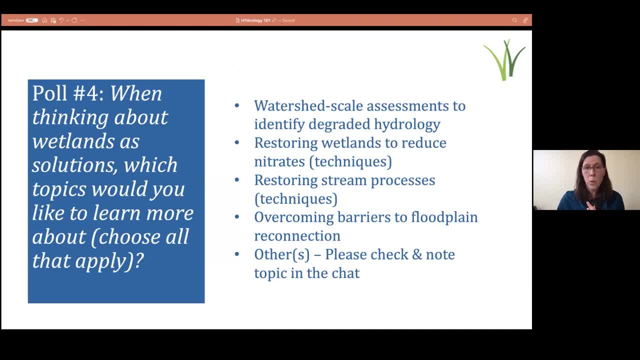 more about And you can choose all that apply. So, Chris, if you could put that in the chat, pop this poll up And this will be very helpful to us and Wisconsin Land and Water and and DADCAP in a project that we're working on collaboratively. that's going to be bringing a lot. 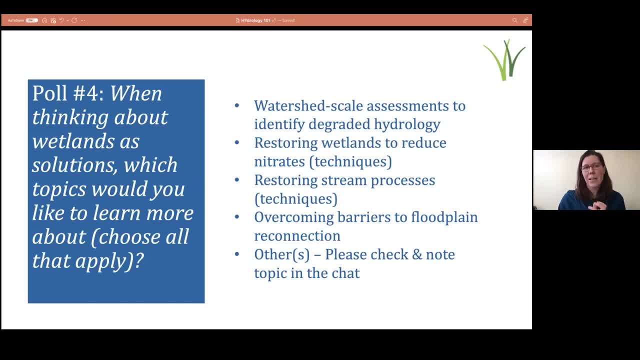 more, more and more detailed technical content and trainings to this audience over the course of the next couple of years. I think, when we close this poll, if, if they're willing- I wonder if we're going to move to questions after this- if either Karine Follett or Matt Woodrow would be willing to unmute and just 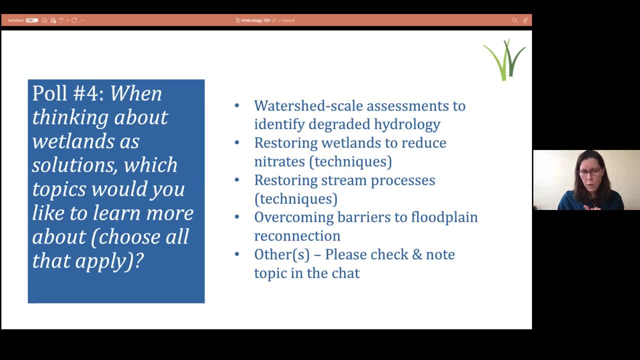 say a few words about the EPA grant collaboration that we're working on and some of its goals, So let's just leave this open for a few more- maybe 15, 20 more seconds. Again, thanks for the engagement. I'm so pleased to see that we have more than 200 people on the call. This is one of the benefits of going. 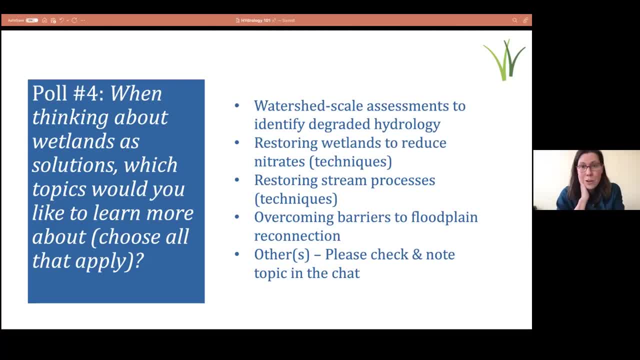 virtual and having no concurrent sessions that we we have a chance to all be here together hearing and thinking about the same content. So lots of interest in how do we do assessments to identify degraded hydrology. Lots of interest in wetlands for nitrate reduction. 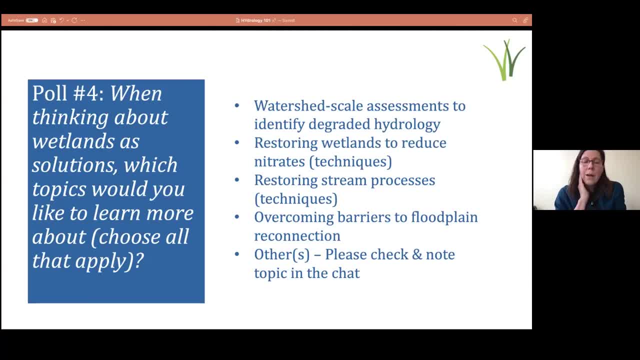 Lots of interest in restoring stream processes. Oh, overcoming barriers to floodplain reconnection- Us too, We're working a lot on that, from both the policy and regulatory and economic side frame. There's there's a lot of issues there that we're aware of, Okay. So thank you all for participating in that poll. Really great feedback. 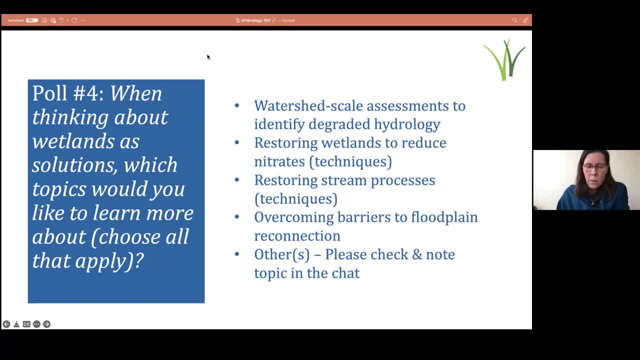 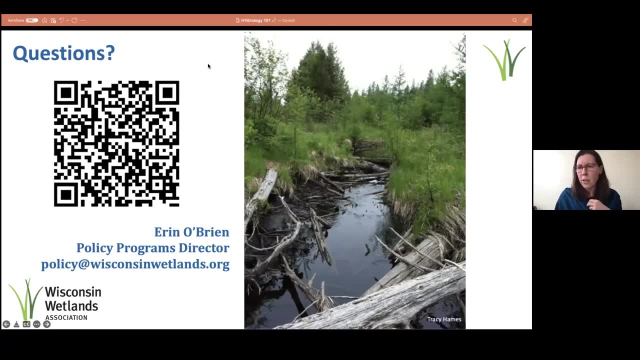 Thank you. So with that, let's move on to some more questions. And for those of you that are looking to get continuing education unit credit for this session, there's your QR code And I'll just leave this up on the board. And if we could, Matt or Corrine, I wonder, could we kick off this discussion? We've got about five minutes left with a few words about the EPA grant. Would one of you be willing to unmute and say hey. 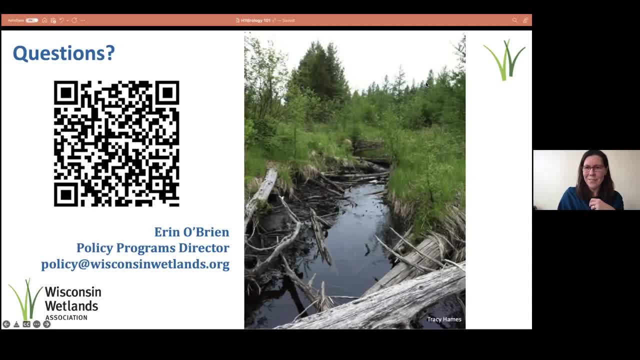 Sure, Okay, Hi everyone. One question, Okay, thanks, Do you want to take the question, Erin? No, go ahead, Corrine. Okay, Hi everyone. This is Corrine at DATCP And Erin. that was a great presentation. Thank you so much. I learned quite a bit, which is good because we are working on this grant together. 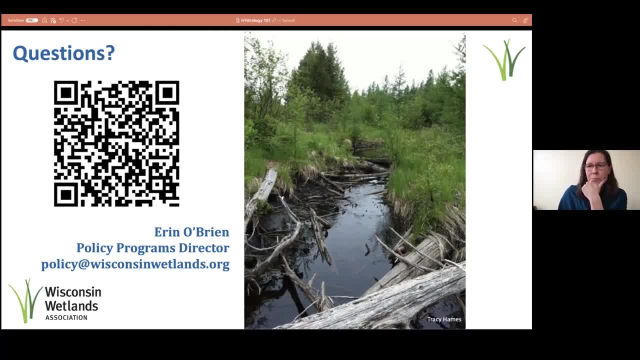 And it it's. I am really excited about it. Erin laid out a lot of information about the benefits of doing these different practices, not to address one site but to look more at the watershed impact of, and benefits of, these types of practices. But when you look at the rule that we have, you know a lot of those practices may not be cost shareable And the timing worked out well. where we are in the process of, we have an open rule and we can consider how we might want to make changes to the rule to better facilitate the grant. 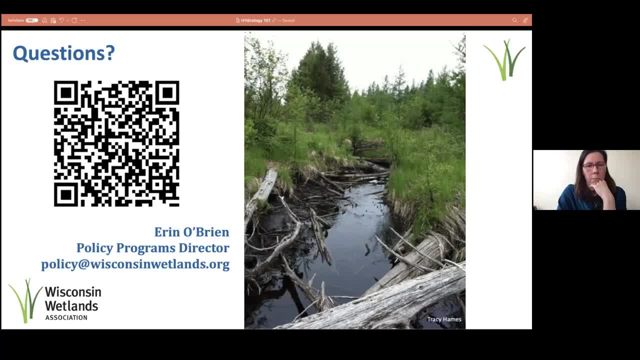 And so, you know, one of the objectives of the grant is to do some analysis and see what types of opportunities there are to incorporate some different practices into our rule, so that you have those tools in your toolbox And then also just doing a lot more training. And we have, you know, Matt and Drew and the other engineering. 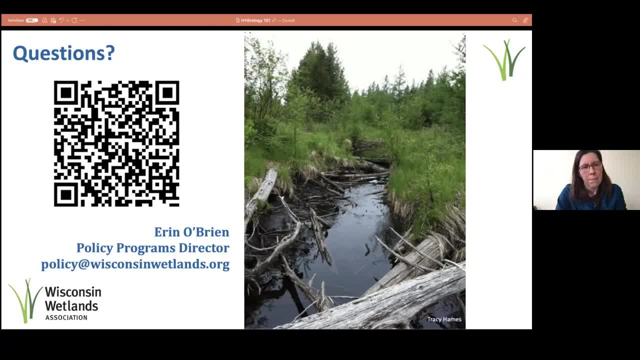 experts are going to be learning more about this at the same time as you all and providing some additional training on this, which we will have more information about as we get further along in the grant. So big picture right now, But I don't know if Matt's on, if he wants to say more about that. 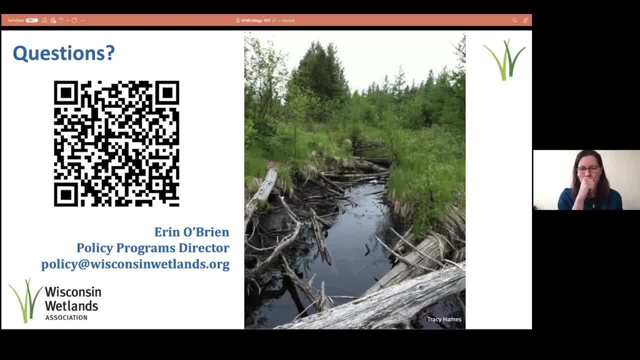 I am here. Thanks, Green, That was a. that was a great overall description of it And, yeah, I'll just touch on the training part of it. You know, like you said, the goal is to get some of these practices into ATCP 50 so they can be cost shareable. But then we understand that there is definitely a need. 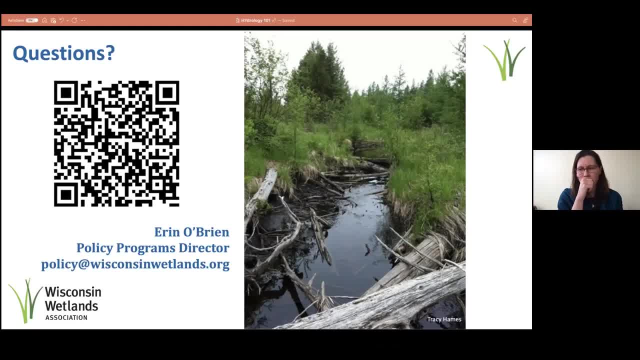 to train on how to identify the right locations to install these practices, And you know, that's something that we don't have a lot of experience in, So we're working to get our staff up to speed on a lot of that. We have a lot of staff that do have experience in that already, So looking to set up trainings to get this knowledge out there as well as part of this. 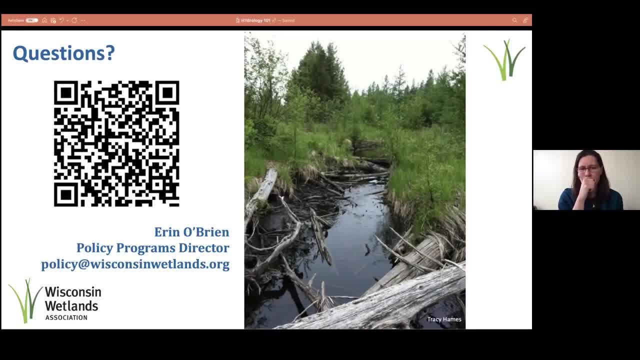 this grant and this, this study of policy. Thank you both, And I'll just mention another area, And then I think we'll have time for at least one more question. Another area that we're working from a policy perspective is that there is 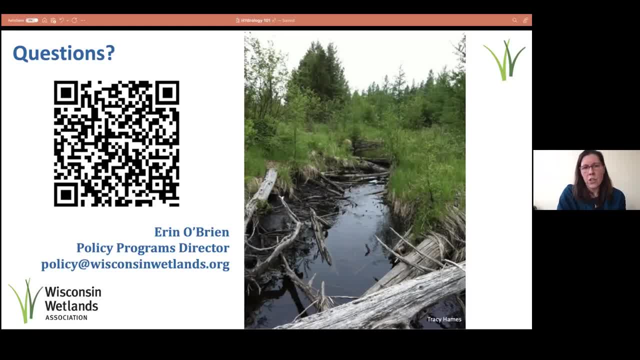 under development. now, as a result of some legislation that passed last session, the Department of Natural Resources is working on development of a general permit for hydrologic restoration practices And the goal there is for the practices that are sort of you know that are sort of you know. 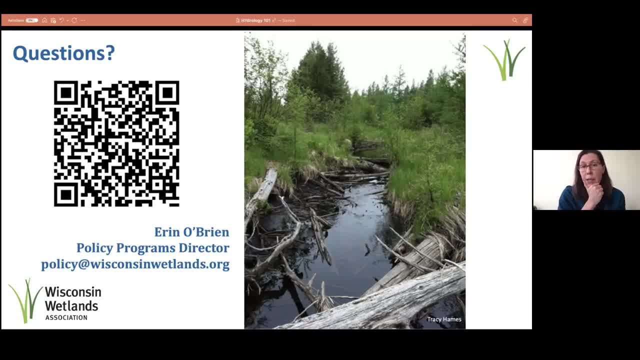 outcomes based to be eligible under GP coverage. So we know there's a lot of- there have been a lot of barriers, perceived or real, to doing work in some of these more sensitive systems, like if you have a degraded trout stream or or or an area where restoration is needed but there's some remnant high quality wetlands there. It's been a little harder to get regulatory approval for those practices. 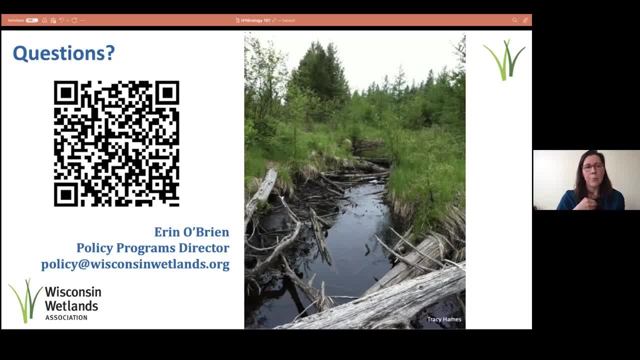 Floodplains is another example And we're trying to move through those conversations of what we need out of our regulations. So we're trying to move through those conversations of what we need out of our regulations to make it a little easier or certain to do that kind of work efficiently and cost effectively. So I think we might have a minute left for one more question, Megan. 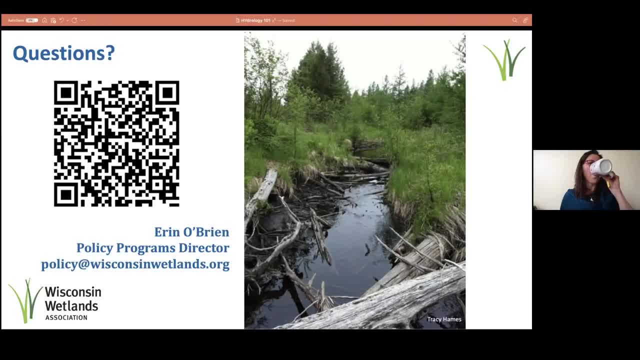 Yep. Um, so what land management techniques which wetlands or wetland characteristics are benefit from grazing and or burning or other management techniques? Yeah, I mean. an easy answer to that is: anywhere where we have, you know, a wetland management system. 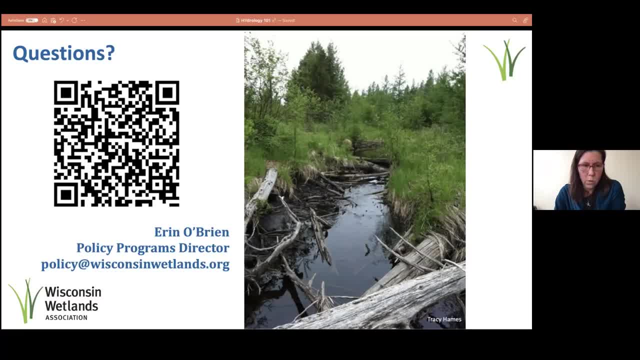 We have overgrown. you know sort of weedy reed, canary grass, phragmites, you know. anything that's in need of vegetation management is going to be a good candidate for generically grazing or burning. now, whether it's grazing or burning, or mowing or chemical treatment. 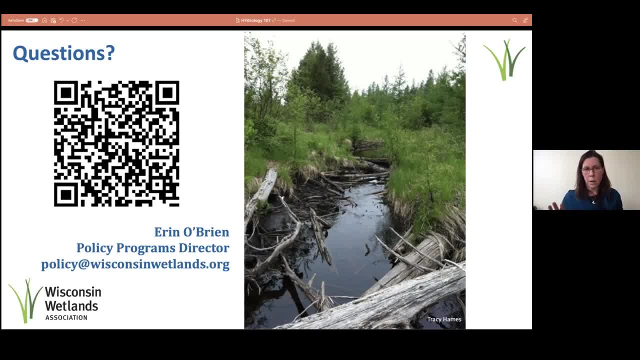 These are all viable management techniques. I'm not the right person to ask about which one you use where, but there's a lot of practitioners out there, A lot of our members, Our wetland managers, that are very experienced in employing all of these kinds of management techniques and others. So it's a matter of really hooking up with the folks that have experienced assessing a given site and making recommendations on which intervention is going to be most effective. 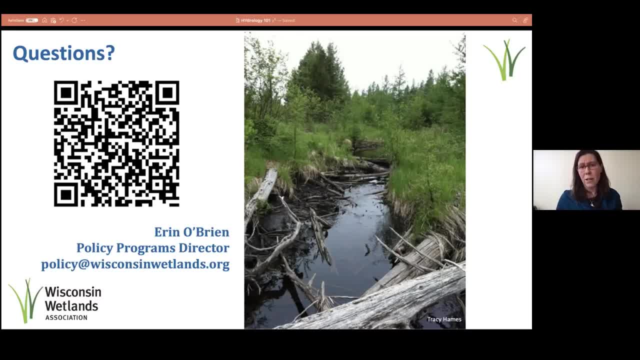 I will say sometimes it takes more than one pass. right, It's really hard to knock back a vegetate- you know an overgrown wetland and it- and it often needs to be used in combination with something else. Right, Some water level manipulation or control to get that hydrology reset so that the